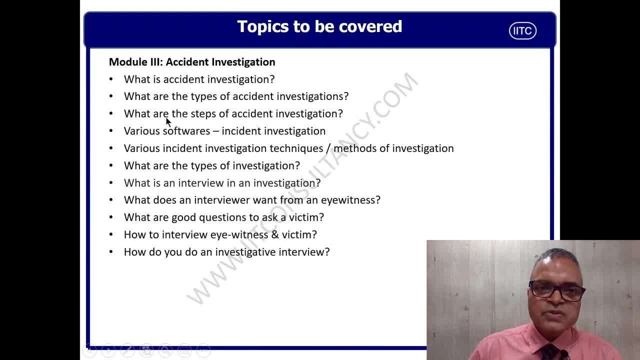 We will see one of them. We will also see what are the steps of accident investigations, What are the various steps, including the ride survey and other things. Various tools, various softwares which are being used for incident investigations. We will only tell the name, Probably we will not go in the detail. 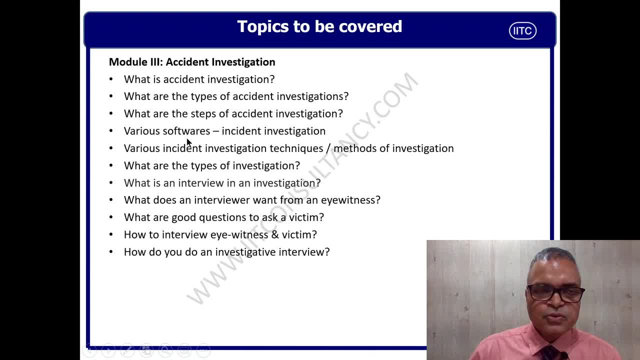 I have different video to help you. which software is best and what are the good softwares, what are the bad softwares And, in terms of my experience, which software is required to use. The incident investigations, as well as root cause analysis for any equipment failure. 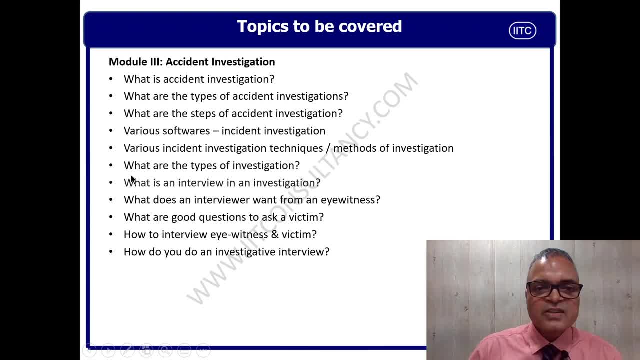 Various incident investigation techniques, as we mentioned earlier. Types of investigations, Yes. and what is meaning of interview? What does interviewer want from an eyewitness? What are the good questions to ask to the victim, How to carry out interviews and eyewitnesses And victims, And how do you do an investigative interview. I hope this is going to use and 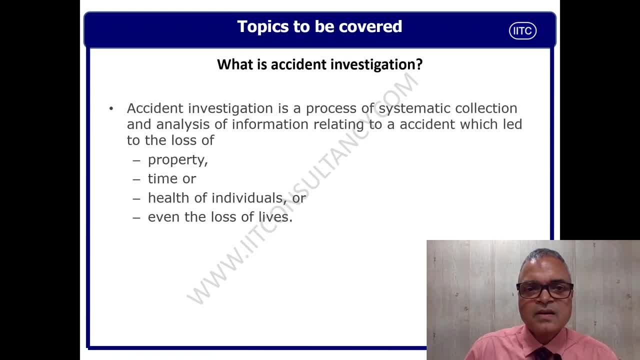 helpful for you. Let us go for the next slide, Guys. now we are going to see what is the accident investigation. In fact, if you see the formal definition, accident investigation is a process of systematic collection and analysis of information related to any accident. 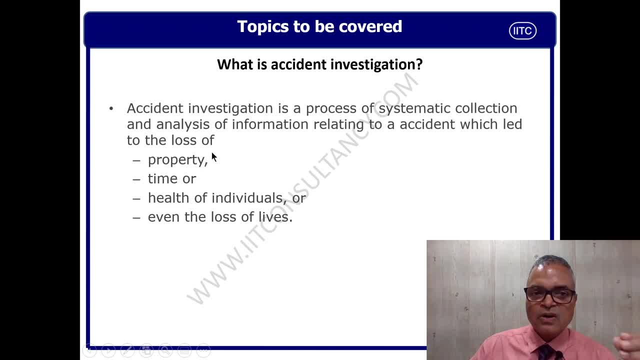 or incident Which has Converted or produced loss of property, time and loss of health of individual, or there is an injury or loss of lives or all together. So this is a systematic process to analyze the data, to find out the root cause. What went wrong, What are the responsible causes? 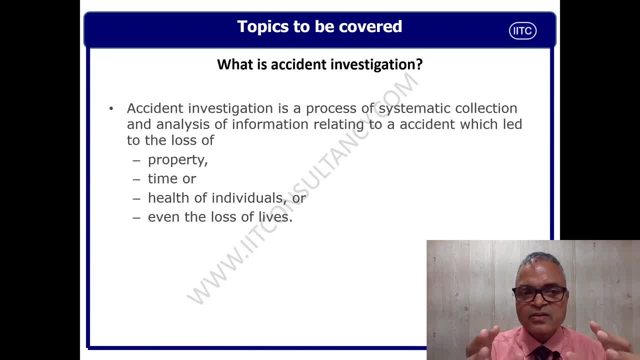 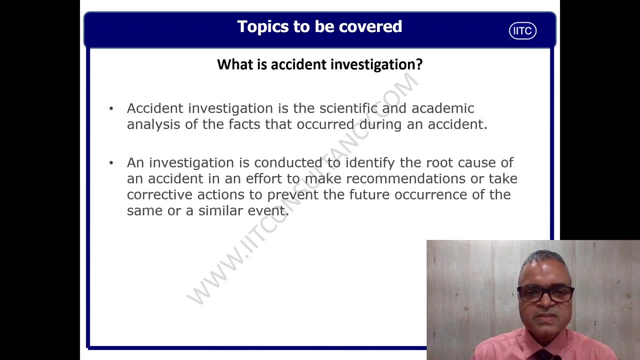 What are the direct causes, What are the indirect causes for loss of life, loss of property, injury, health effect or all of this? Probably, in the following slides you will understand clearly what do you mean by incident investigations, As we know that accident investigation is basically. 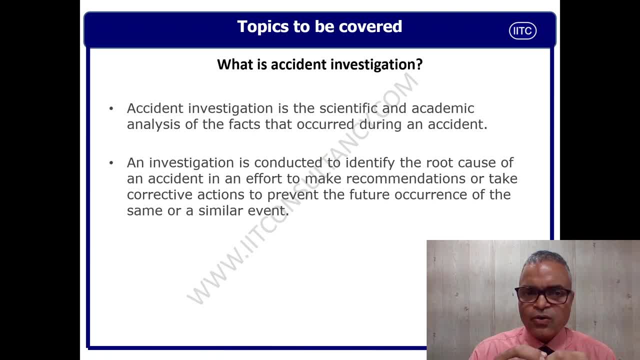 a scientific and academic analysis of all the data, of all the facts, what has been collected after the incidents, Site securing and what has gone wrong during the incident, to find out the root causes of an accident, in effort to make recommendations or take corrective actions. The ultimate aim is to find out the root cause is to prove to implement these. 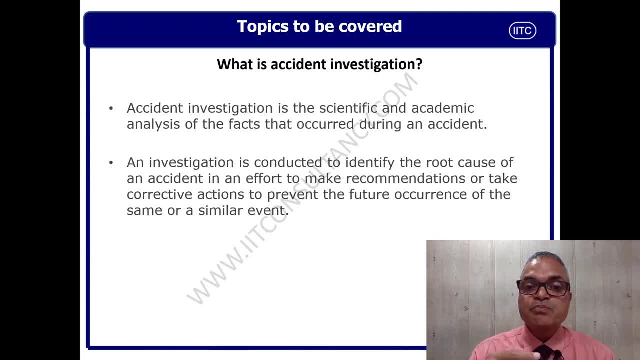 root causes so that we can stop, We can prevent the- I mean reoccurrences of this kind of similar incidents in future. So the ultimate aim probably? there are some slides which will tell you the intention of accident investigation, But for now we can say that accident investigation is to be done to find out the root causes. so 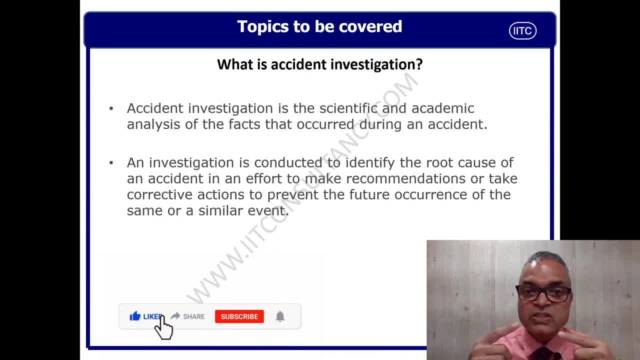 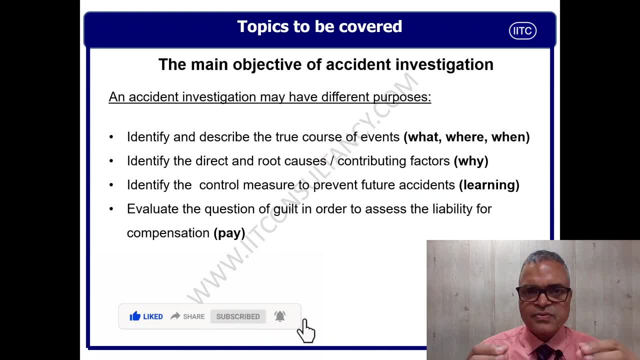 that we can implement it and we can prevent the reoccurrences of this kind of accident. Guys, if you see, the main objective and purpose of accident investigations are many. You may be knowing it, But to summarize the crystal clear, I mean intention and the purpose of 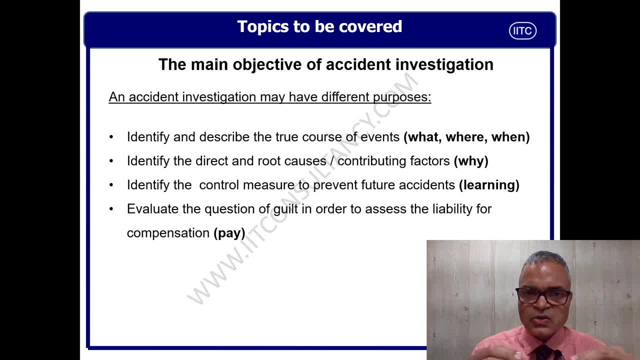 accident investigation is to find out the root cause of the accident, The root causes of an event in this, what has gone wrong, where it has gone wrong? when it has gone wrong, we will see it. And the second is to identify the root causes or contributing. 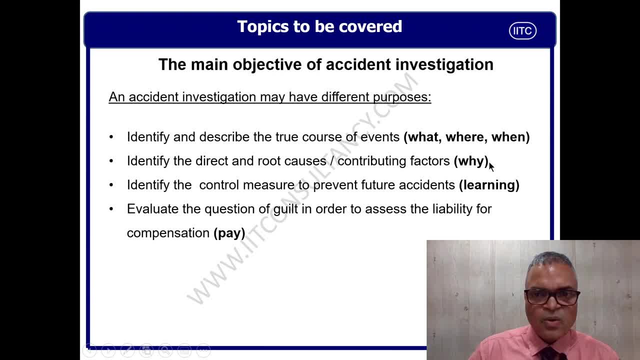 factors Why this incident has happened. What are the system failure We will try to identify in step number two. Then the next purpose of the incident investigation is to find out the control measures to prevent the reoccurrences of this kind of incidents. 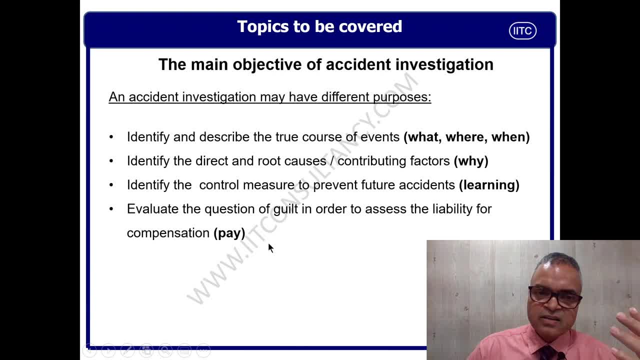 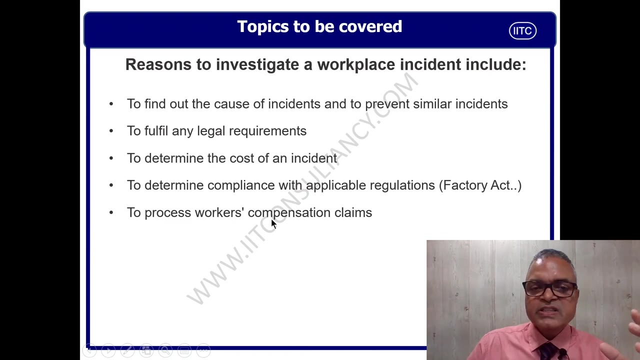 In future, this may come in the learning phase and definitely evaluate the questions of guilt in order to assess the liability of compensation, Because if there is a partial damage or partial permanent disability, we need to pay the compensation as per the compensation workmen compensation act. So, if you see, and the reasons to investigate workplace incident. 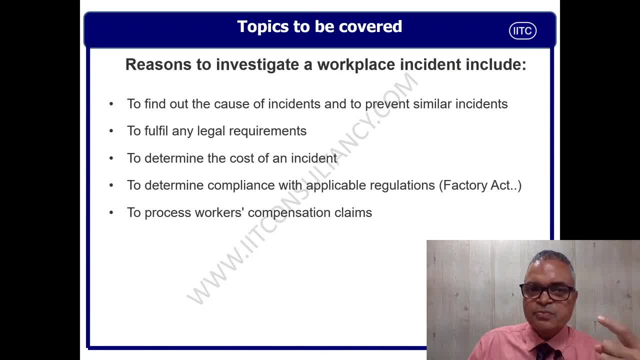 Those are very much similar to the purpose. The main and foremost important reasons are, or reason is, to identify the causes of accident, to prevent the similar incidents in future. Second reason is very strong reason. It is one of the legal requirement as per the factory act, Indian factory act. 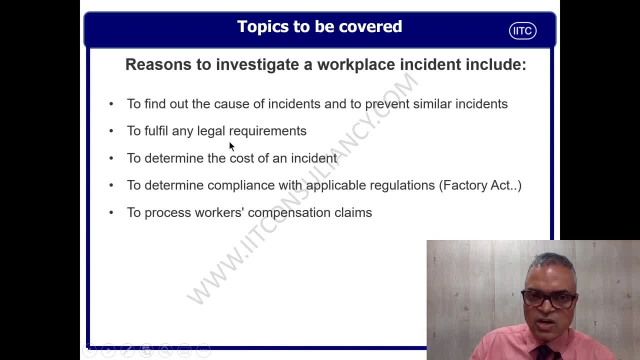 Likewise in India. there are many countries where legal requirement says that each and every accident must be analyzed, must be investigated, to determine the cost of an accident. Sometimes many companies also want what cost has incurred or occurred during this incident. There are direct cost, there are indirect cost, which we have seen in other presentation. 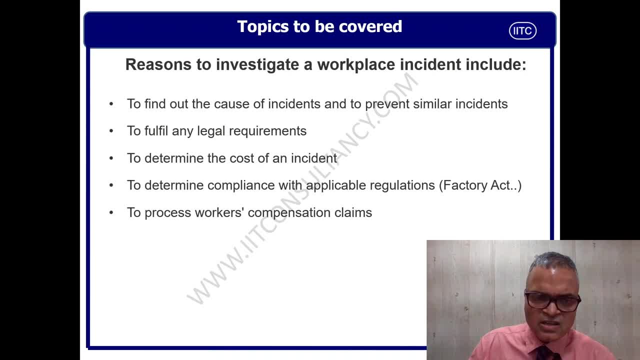 of safety transformation. I am not going to repeat what are the causes, what are the cost of incident, whether this is direct cost or indirect cost, But we can say that this is one of the reason or one of the requirement to determine the cost of accident. 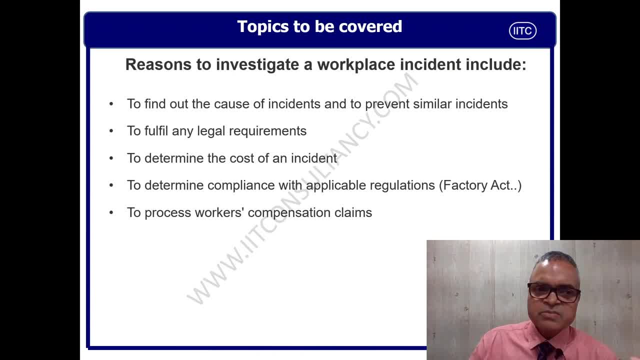 That is why we need to do the incident investigation, So sometimes determine the compliance with applicable regulations, like factory act, like environmental pollution control of pollution prevention, And there are many more regulatory requirements. are there? Probably it is not. it is difficult for us to tell you now. there is one presentation. 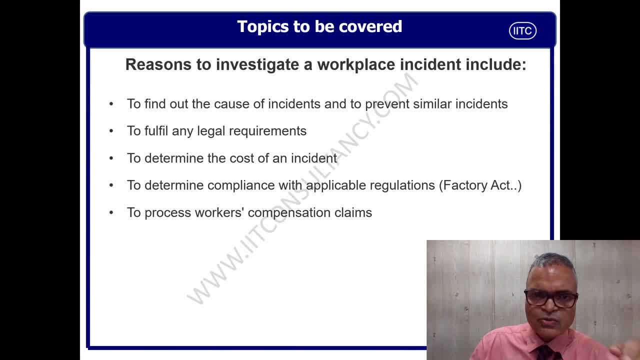 what we have published to identify And why legal requirements are there and which kind of legal requirements are there to identify or investigate the accident, to process the worker compensation claim- Because, as we know that there is workman compensation act is there- and to identify what is the permanent. 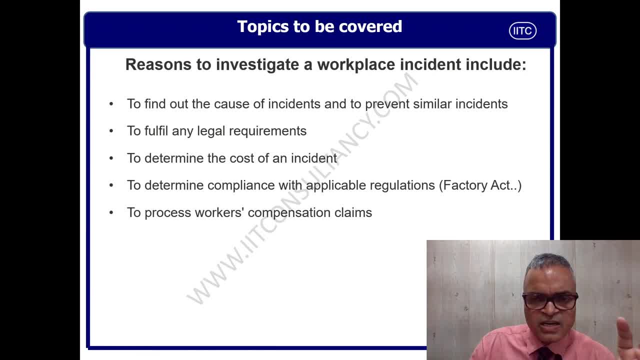 whether there is a permanent damage or there is a temporary damage. there is permanent partial damage or permanent full damage. There is a partial full damage or partial temporary damage. This is the workman compensation act requirement And this is why there is a need for doing the incident investigation to find out the 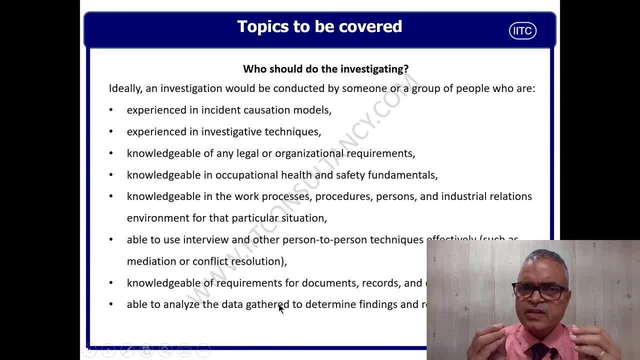 root causes for that. Guys, now the very important thing is who should be part of incident investigation. Basically, incidents are to be conducted by group of people who has got some definite, definite attributes Like. the person should be knowing the caution model. He should be aware of incident investigation techniques. 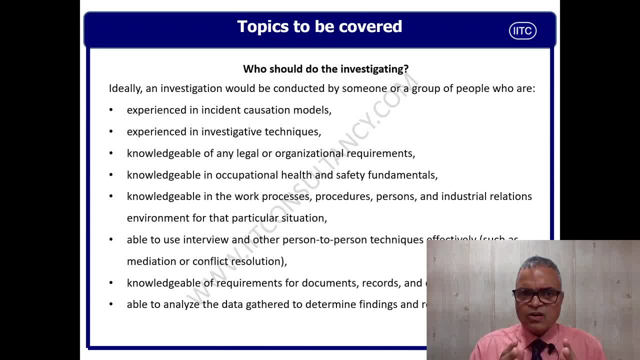 The person should be knowing the caution model. He should be aware of incident investigation techniques. The person should be knowing the caution model. The person or one of the team members should be knowing the legal or organizational requirement because he has to find out what are the legal requirements and what are the rules and regulations. 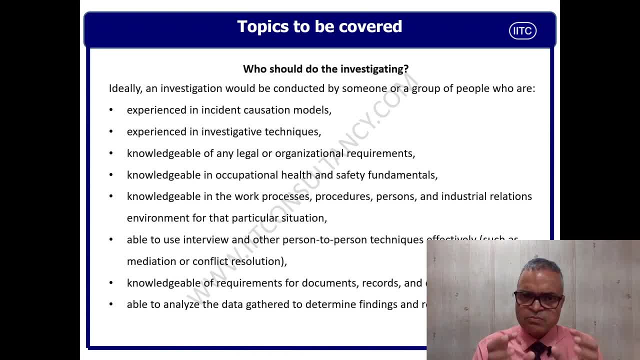 And he should be- definitely he should be part of or he should be member of, occupational health and safety fundamental situations. The person who is doing the investigation: he should be knowing the occupational health and safety management systems or safety management system. The person who is doing the investigation: he should be knowing the occupational health. 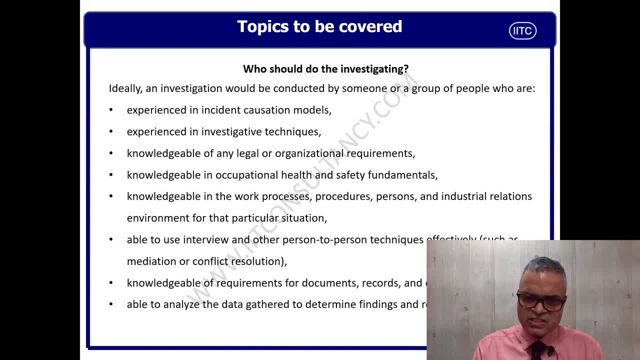 and safety manager system or various elements of Safety management systems. We have seen safety management system separately in earlier presentation. probably I will request you to please- I mean go through the separate individual safety elements. There are 15 safety elements and they should be a part of the safety management system. 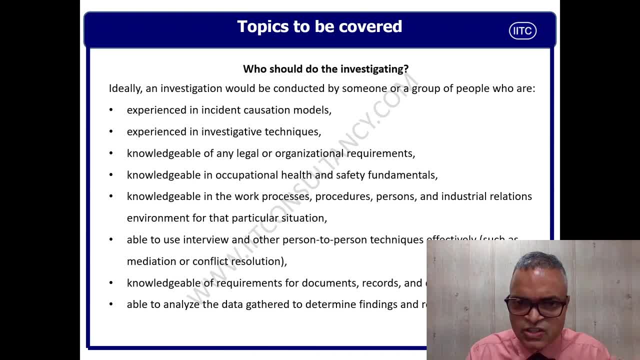 And we have published a very important ah ah elements of of the entire safety management system. as per your convenience, I would request you to. if you have any question, any suggestion, please feel free to put into the comment section so that we can come back to you. and, very important thing is, if you have not subscribed the channel, 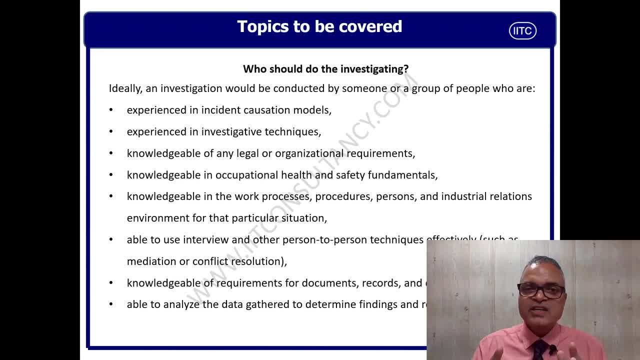 so far. I will request you to please subscribe the channel so that you can get a regular and update on our new publications, new videos, new updates. and the person should be knowing- I am NOT saying one person should be knowing- the member of the investigation should be knowing the work, processes, the work. 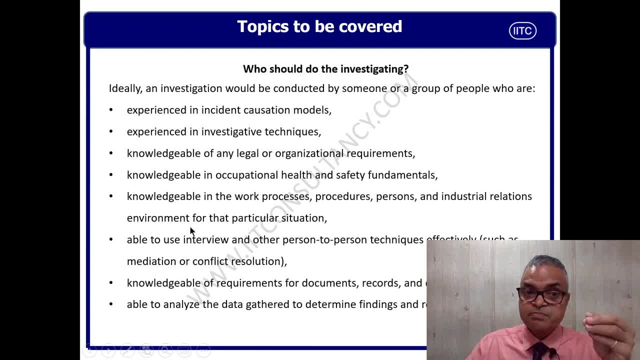 procedures, persons and industrial relationship, working environment. and the person should be knowing the interview techniques because interview is one of the important, vital element of doing the investigations. and the person should be doing unbiased, neutral, nodal interview so that he or she can get a concrete root causes analysis. so the person or 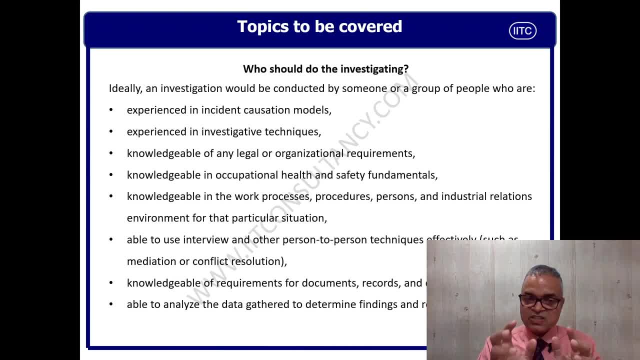 you investigation team. one person of persons should be knowing the different interview techniques to interview, eyewitnesses to interview and the victims the interview, the other related persons, their interview maintenance person of person, people, legal persons and many more, and the person or team member should be knowing it. requirement of documents, records and data collections. 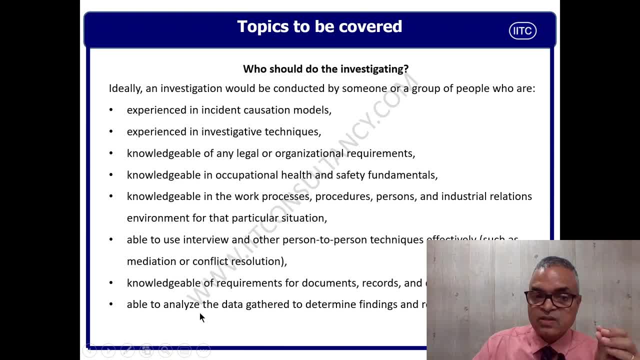 definitely the person or the team should be knowing how to analyze the data, get a gathered to determine findings and reach recommendations. The ultimate goal is to find out the real root causes for the incident and to give the concrete, solid, smart, specific, measurable, achievable, reviewable and time-bound recommendations. 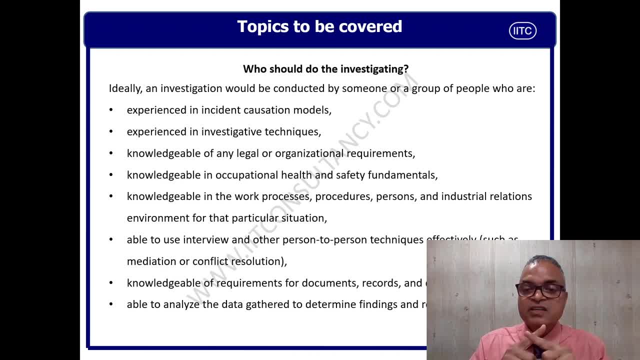 so that these recommendations can be implemented to ensure this incident does not occur in future. Guys, I hope you understand I am going little fast because I want to give lot of information in given point of time. If you have any questions, please put in the comment section of the channel so that we 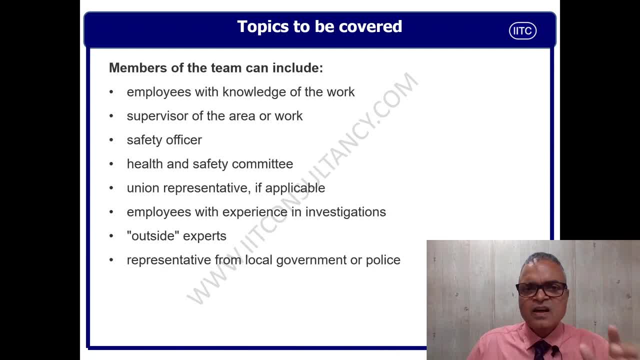 can come back to you as early as possible. Typically, the members of the investigation team should include employee who is knowledgeable of the work, So one person should be knowing what work was going on and how the work is done. What are the hazards? what are the normal hazards in the work? 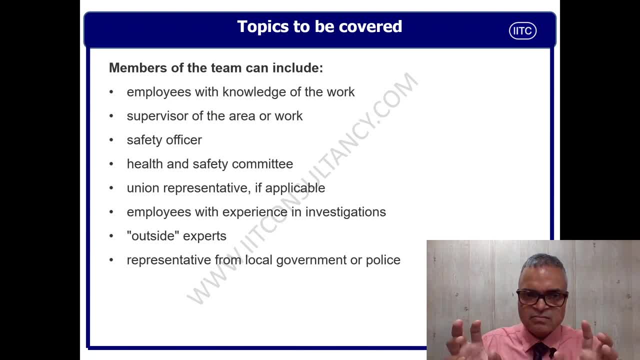 He should be familiar with JSA. The supervisor of that working area must be part of the interview because he is in charge. he knows the psychology, he knows the working environment. he knows the personal behavior. he knows what are the unsafe act, unsafe condition. he knows the JSA. 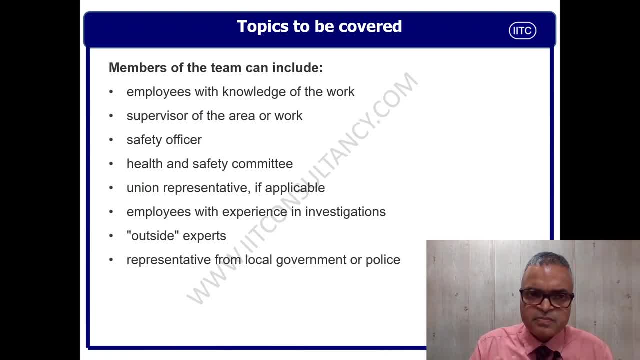 The supervisor must be there during the interview. Safety officer: one person from the safety department must be there. he should be familiar with all safety requirements, all legal requirements, all specific rules and regulations, acts and regulations. Safety committee meeting team should be there. one person from the safety committee should. 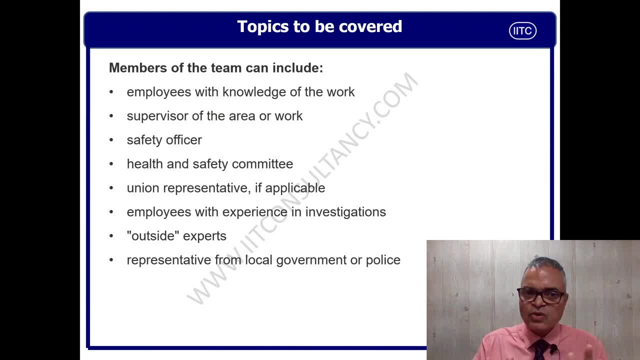 represent in the investigation because he or she is knowing our safety committee requirement and he and she should be able to demonstrate in the next safety committee meeting how the investigation was done, what were the root causes, what are the recommendations, how the recommendations are being closed. 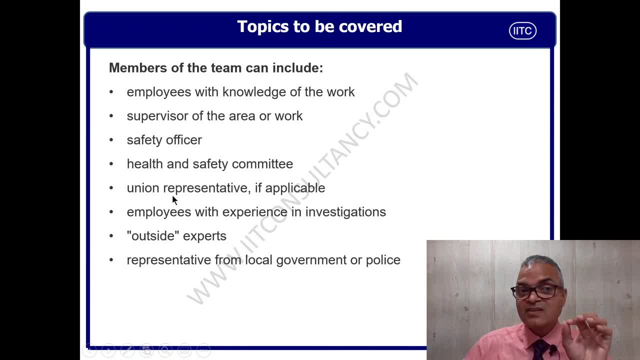 Definitely union representative must be there. because the worker representative from the union should be there? because there are some legal requirements sometimes. if there is no legal requirements, definitely some someone from the worker representative should be there to ensure that worker or team points are well considered during investigation. 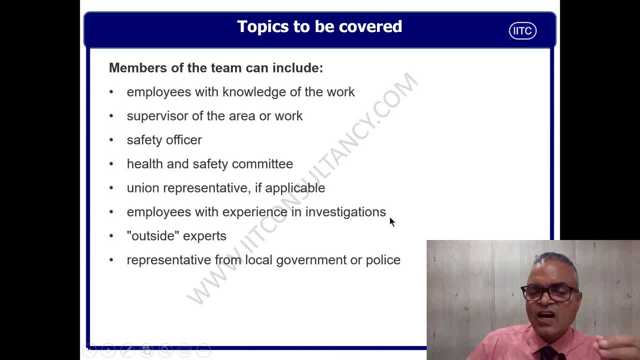 Employees with experience in investigations, as we mentioned earlier, that the person or the team should be knowing different techniques, different steps of investigation and, of course, sometimes outside expert. what is meaning of outside expert? that means those technical person who is not working in the organization. he should be hired from outside as a third person point of view or as a 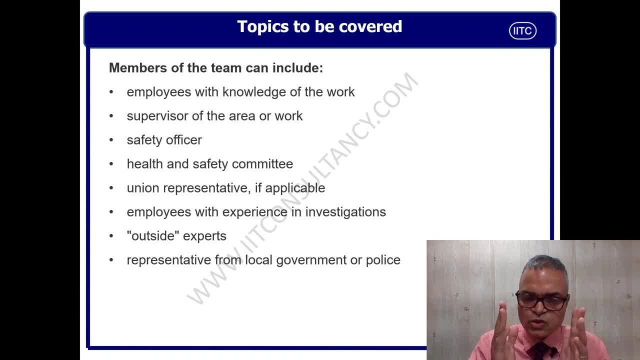 bird eyes point of view, because you are the expert, you may be knowing everything. probably you are complacent. you are not able to see the risk or hazards of the incidents. so that is why we need to take the input and the technical aspect from third party investigators. representative from. 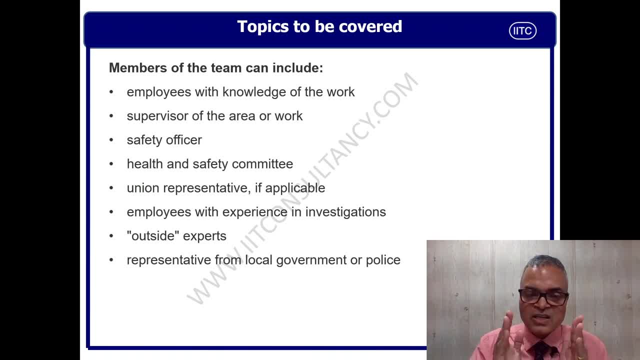 local government or police. sometimes it is requirement of police, requirement of legal document, legal legal authority to participate. so these are the minimum structure of investigation team. depending on your requirement, law of land, police requirement and your company philosophy. please construct or constitute, or i mean investigation committee who can. 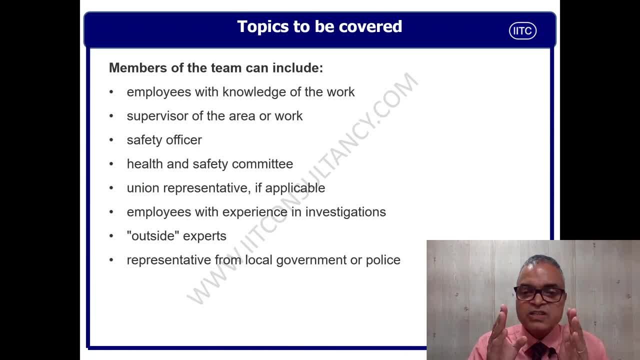 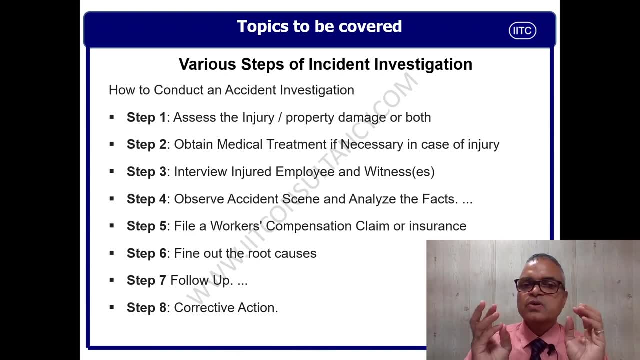 do on or participate in incident investigation. guys, now we are going to see the various steps of incident investigation, how to conduct a very constructive fool fool, foolproof investigation. there should be some series of steps, what we must know. the step one says that assess the injury, oblique property damage or both. 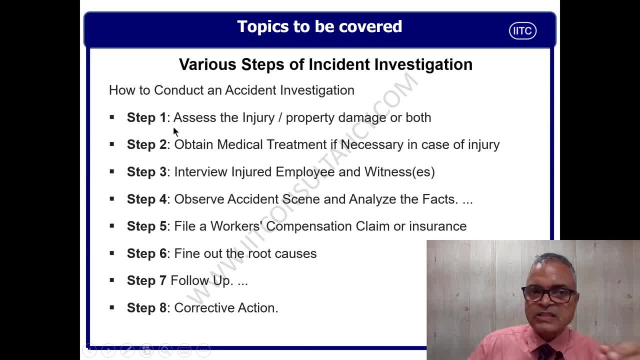 we will take these steps in detail how to be done in- i mean following slides. she can obtain the medical treatment if necessary in case of injury. then third step, interview injured employees and eyewitnesses how the interview is done. what are the different aspect of for interview? what are the do's and don'ts of interview? we will see separately, observe accident scene and analyze. 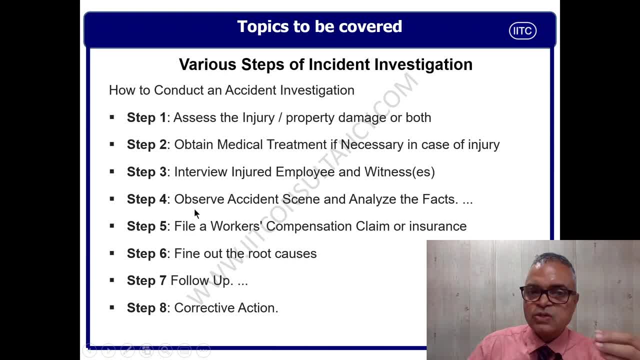 the situation and then we will take the photographs and the data from the incident place and we need to gather the data from the incident place. we also need to take the photographs in sequential manner so that at latest stage we can do the investigation to find out the correct root cause and fact finding. 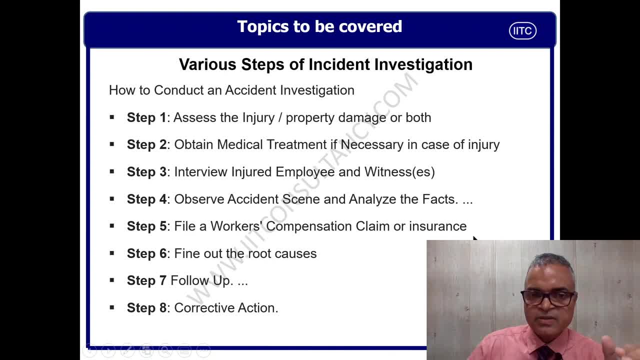 file a worker compensation claim. definitely. i mean, as per the indian rule and as per other country ruled, there is a workman compensation. so after that we need to file a workman compensation claim or insurance. find out the root causes. we need to find out the root causes of the incident. 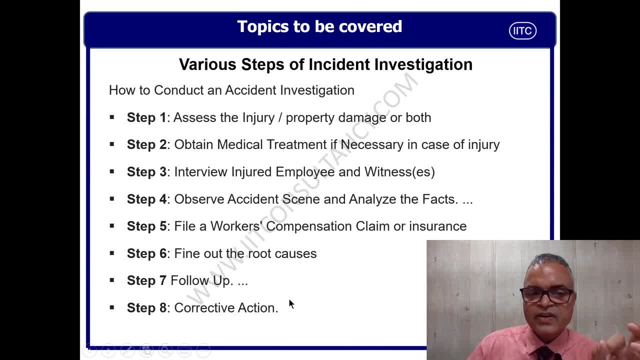 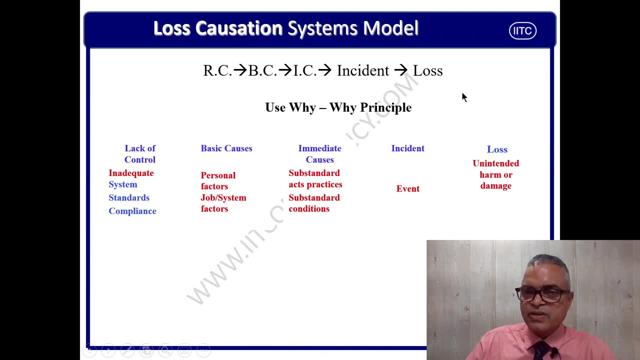 then we have to follow up, uh, the root causes and definitely the corrective action has to be identified. and after character action is identified, corrective action has to be implemented to prevent reoccurrences. guys, here we will see a low scotion system model very quickly, i will not take much. 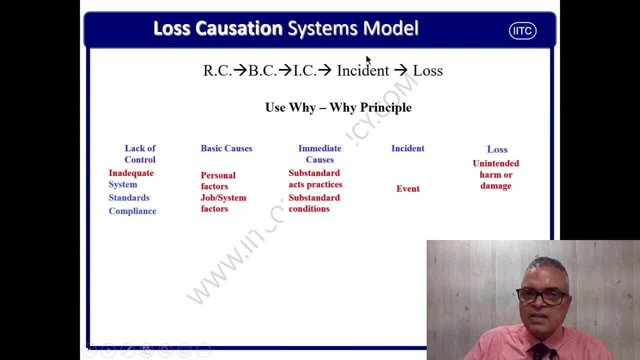 time of yours here there is a loss, then incident, and then we have to identify the root causes of the incident. then immediate causes, basic causes and root causes. this is the sequential process as per the caution model. so before behind a loss there is incident and behind any incident there is a immediate causes. 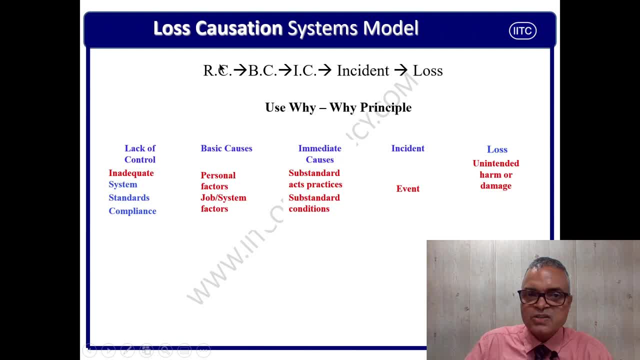 and behind, uh, this thing, there are some basic courses, then root causes. let us understand with this- i hope you are able to understand and see my cursor- there is a loss which is unintended or damage. this has happened because of an event. this is the unwanted event means incident. 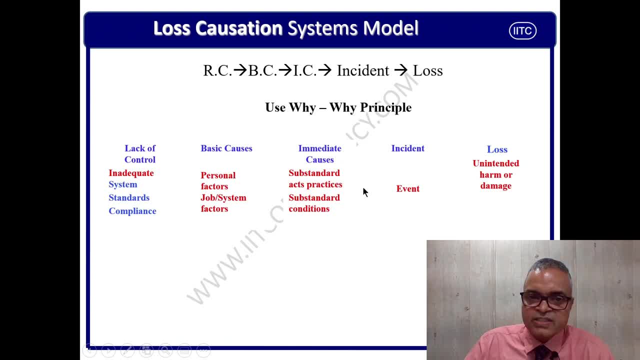 the immediate causes may be substandard F or conditions that we need to identify the basic courses, may be a personal factor or job factor factor or system factor or organizational factor, and then we need to find out root causes. basically, this is the management system failure. we will see how it is going to implement, how it is going to be effective, in the following: 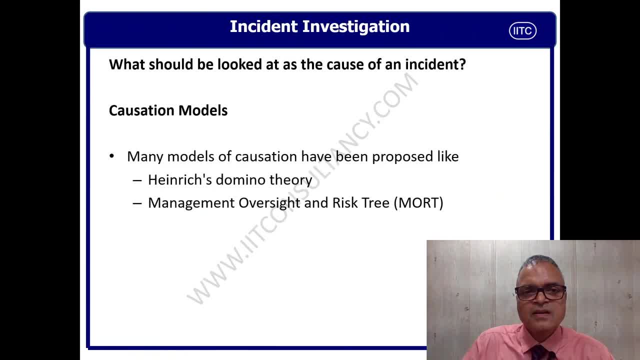 slides to understand. to explain you very clearly, guys. now we do understand what should be looked when you are doing or identifying the cause of an accident. basically, there are various caution orders are there and we are going to see Henry's domino theory, as well as management of management. 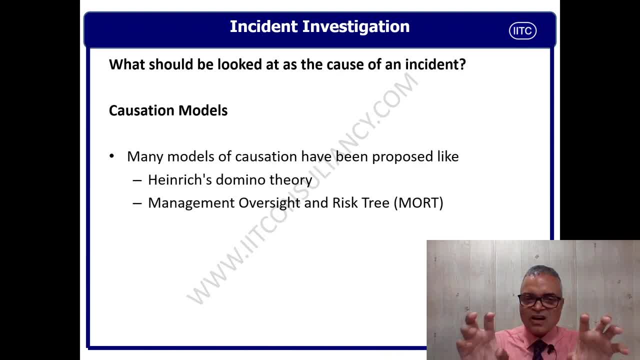 oversight and risk tree. this is the different methods of incident investigation we will see in the following slides very quickly, so that you can clarify your doubts. if, in case of any question, I will request you to please- I mean, put your query in the comment section so that we can come back to. 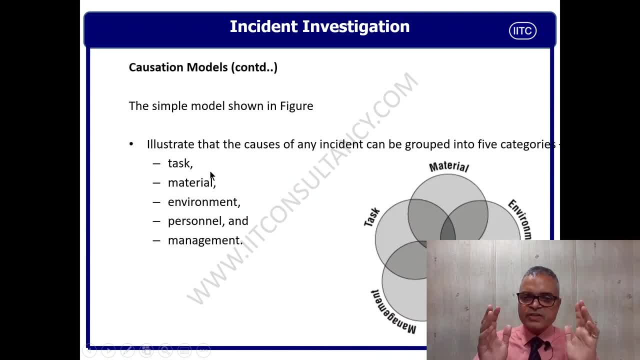 you guys, if you see, this is the simple model which has been shown in the figure on the right below. there is a contribution of the causes from the material side. there may be causes from the environment side, there may be causes for personal side, may be management side or task side. so we 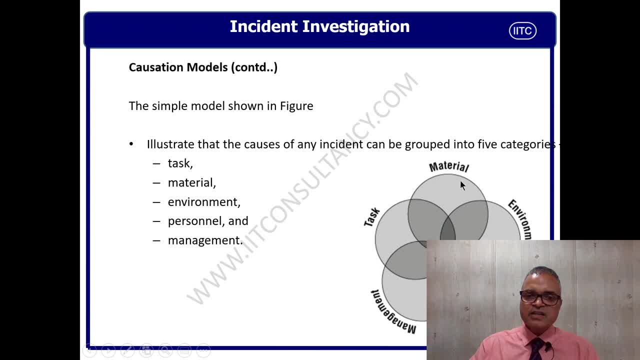 will see everything one by one, from task, from material, from environment, from personal and from management perspective, so that each point can be clarified to you, so that you understand the aspect of incident investigation and real techniques of incident investigations. I hope this slide can clarify you lot of. I mean queries and doubts. if you have any question, please put in the comment. 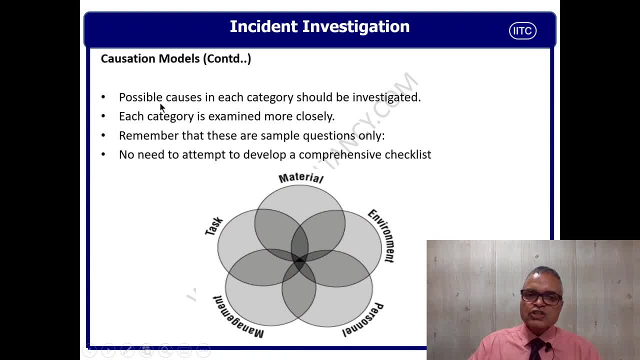 section so that we can come back to you. possible causes in these categories must be investigated, beginning from the task: material, environment, personnel and management. Remember that these are the sample questions only. There are some questions in the following slide, but these are the sample questions. 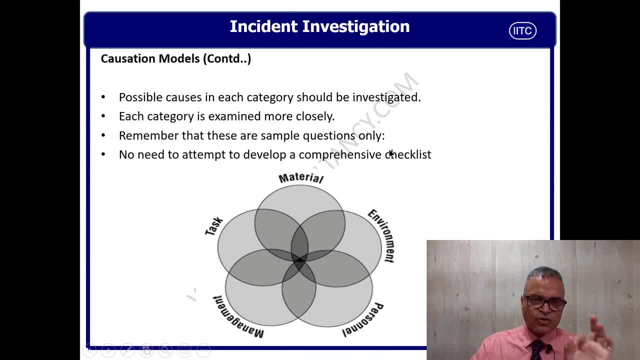 only You can customize these questions depending on your company, depending on your working style, depending on your procedure, depending on your processes, depending on your working environment. No need to attempt to develop a comprehensive checklist. Question is there? are these checklists what you are going to see in the following slides? 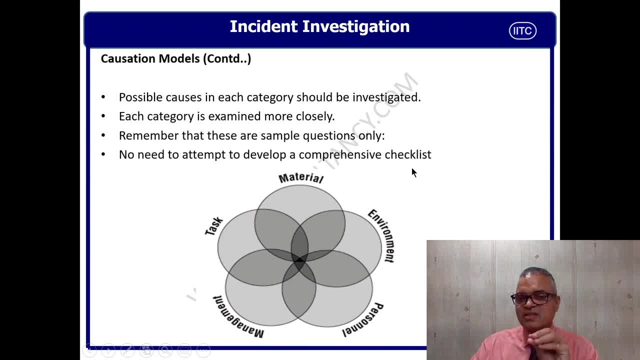 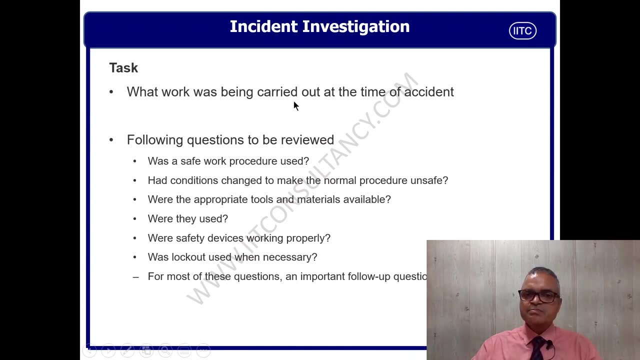 I would say that sometimes you need to check it whether this is effective or not effective. If there is not effective, then you need to probably customize it. No need to make a change of all the questions. Guys, now here in the task. we need to know what work was being carried out or done at. 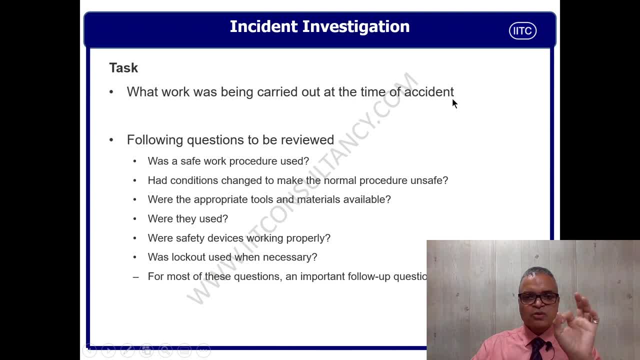 the time of accident. This is the worst and first foremost, important question. Following question must be reviewed. What is the question? Safe work procedure must be reviewed Whether the safe working procedures have identified all the hazard, whether the work procedure has been fabricated or formulated with the help of JSA. what are the unsafe conditions? 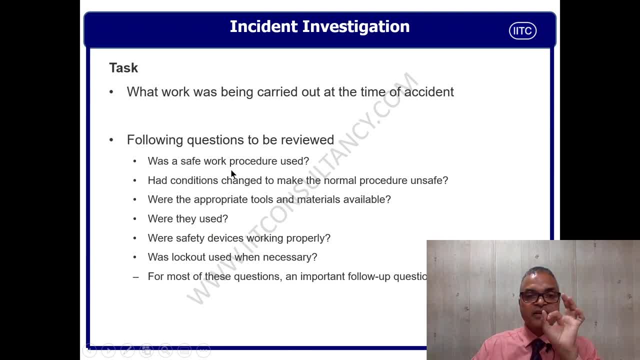 what are unsafe hazards? what are unsafe actions? substandard act, substandard condition. I am going through little fast so that I can give you more information in the given stipulated time. Now we will say that highest condition changed to make the normal operating procedure unsafe. 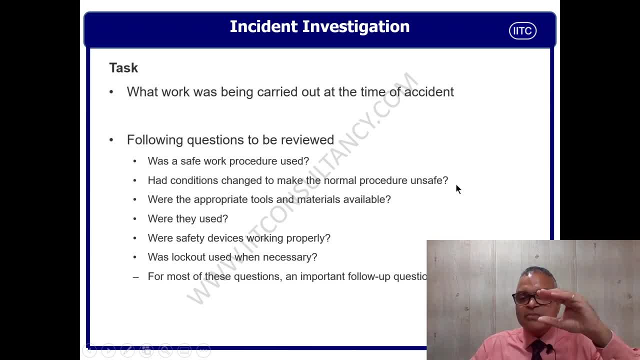 See there, the normal operating procedures are there. but whether there is some change in the condition, in equipment, in the change of machine, change of men, change of processes, Then we have to analyze slowly, slowly, where the appropriate tools and material available. 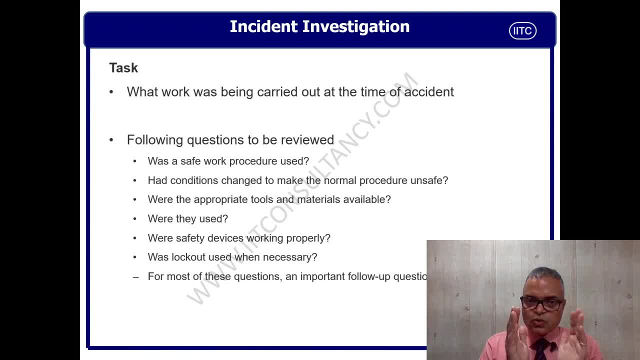 So we need to identify at the time of incident whether correct tools and correct material was used. If they make a shortcut, they use manipulated tools. maybe they are using wrong tools. maybe they are using damaged tools. whether they are using the correct material, maybe they. 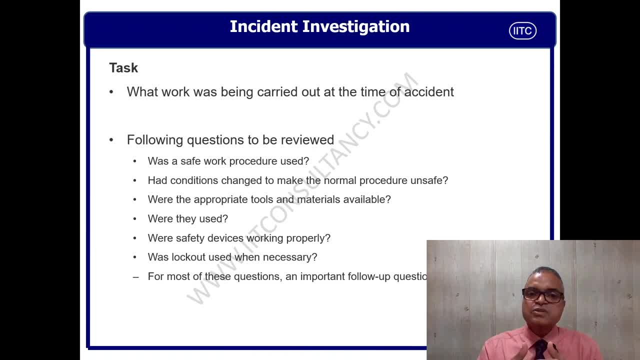 are not using correct chemical to clean the equipment. maybe they are using the different chemicals. So that is why we need to find out where appropriate tools and material was available And whether that materials were used. that tools were used, we need to identify what. 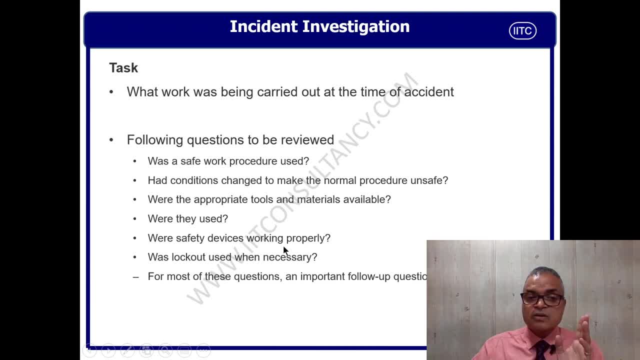 was the safety. We need to find out where the safety devices are there and where safety devices working as per intended requirement or as per intended design was lock out and take out system was used. If, in case of loss of potential energy, whether the electrical permit was used, whether permit. 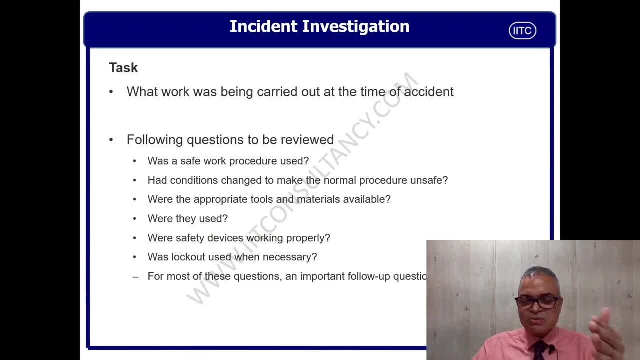 to work system was implemented, whether the people were trained. This we will see. work wise was probably. there are machine material management. these points are another. For most, this question, an important follow up question, is: if not, why not? we must ask. 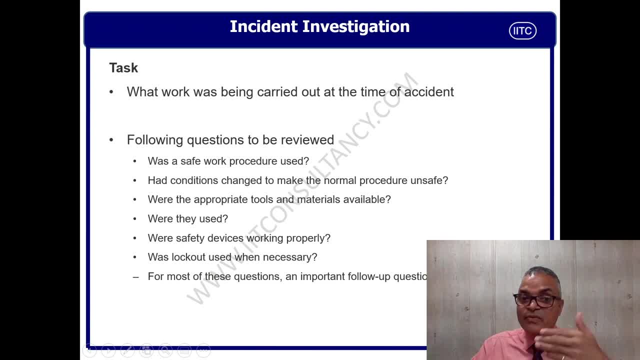 if not this, why not, if this was why this was. we need to keep triggering this thing with a lot of questions with: if not, why not, if yes, why yes? So this will trigger the right answer while doing the investigation. 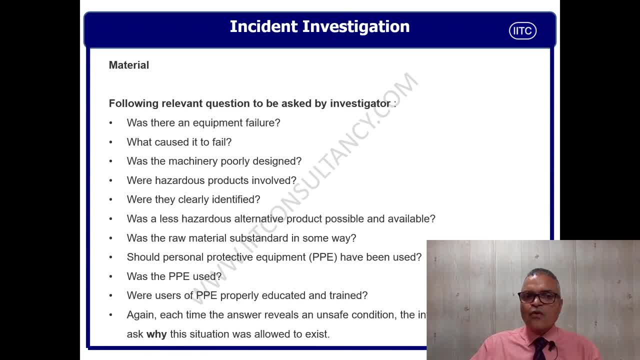 These are the questions related to the machine. I will just go through very quickly: Where there an equipment failure? whether there was equipment failure. what cause to fail this equipment. what was the reason for equipment failure? was machine properly designed? whether the machine which was used to- I mean process the material it is poorly designed. 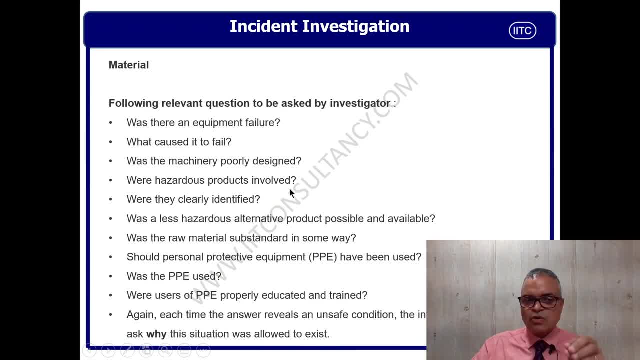 or properly designed Where hazardous product involved. what was the hazardous product? what was the hazardous chemical? what was the hazardous? I mean raw material was used Where, Where they clearly defined was the hazardous product, hazardous chemical was properly identified, properly defined, properly identified the hazards was a less hazardous alternative. 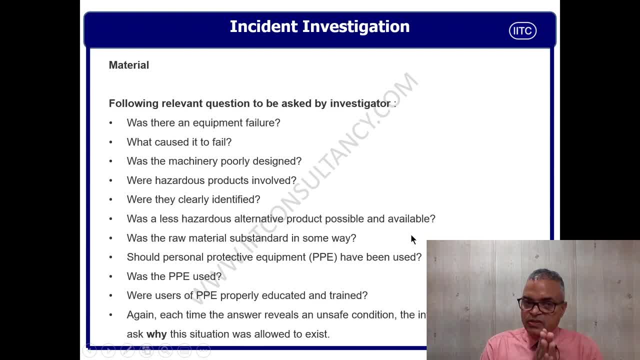 product possible and available? we need to identify if there was use of hazardous material, hazardous processes, hazardous equipment, hazardous raw material. is there any less hazardous product process material is available to perform? So this is the question. Thank you. 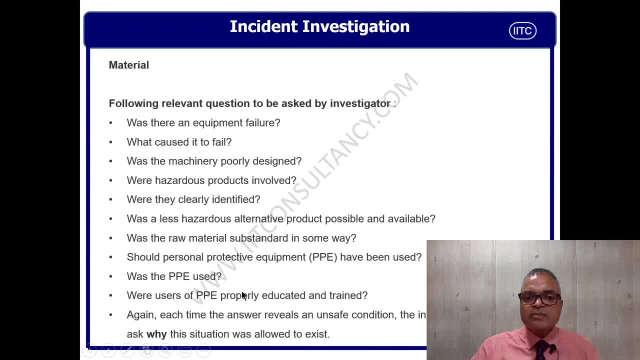 If the raw material was substandard. we need to find out whether the raw material was standard raw material or it was substandard, because sometimes people take deviation, they use less standard material and there is a wrong processes and then there is accident. Should personal protective equipment have been used? whether they were given PPE was. 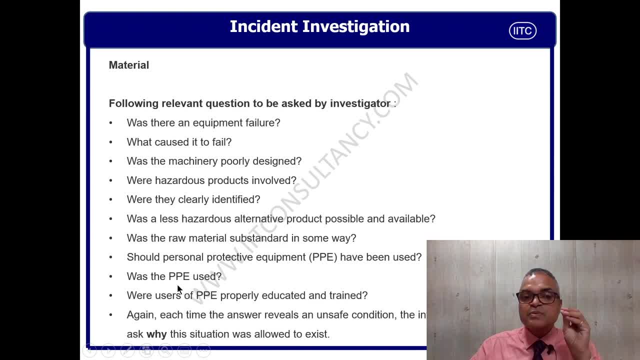 there requirement of using the PPE. whether people were using the PPE where users know how to use correct PPE and how to maintain PPE. whether the people trained about how to use and maintain the PPE. again, each time, the answer reveals an unsafe condition. the 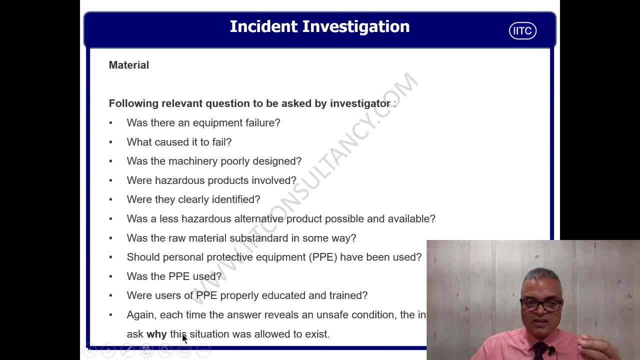 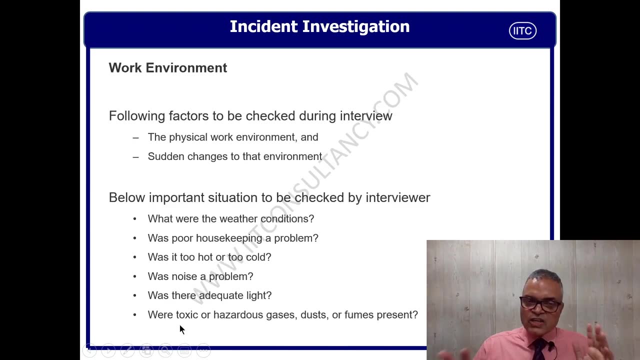 investigator must ask why the situation arises. so, guys, I am going through very quickly, I am again reminding you. please, if you don't have, if you don't, if you are not able to understand, please revisit this video again so that you understand this question and this query. likewise task, likewise material we need. 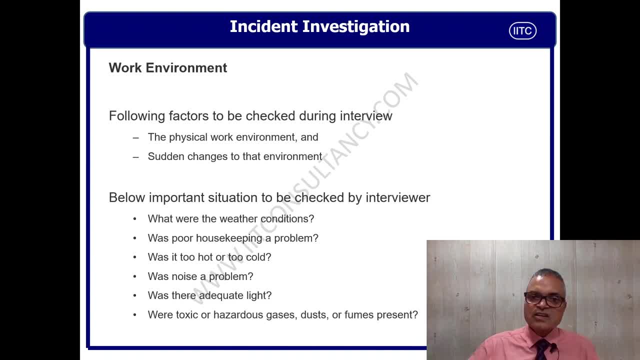 to identify work environment following factor to be checked during the interview: the physical work environment. what was the physical work environment like? temperature, humidity, slippery sleep and sleep condition, electrical condition, And was there any sudden change to that environment? Was all of a sudden air conditioning failed to work? Was there sudden high noise in the working environment? Was there sudden slip and trip or some chemical spill? So this we need to identify while we are doing investigation of work environment. 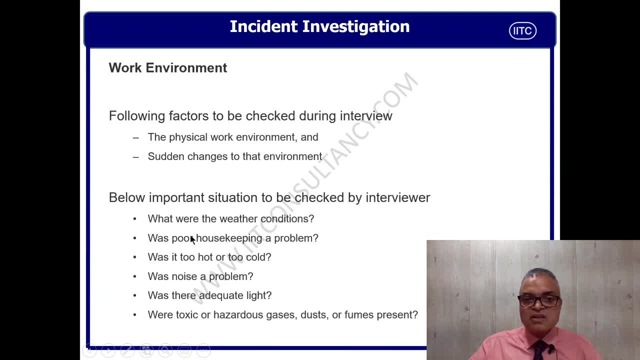 Below. important situation must be checked by interviewer. What were the weather conditions? Temperature, noise, illumination- These all are physical weather conditions. Where or was poor housekeeping there? We need to identify slip and trip slippery chemicals. There are unsafe conditions. Was it too hot or too cold? Temperature was very high. 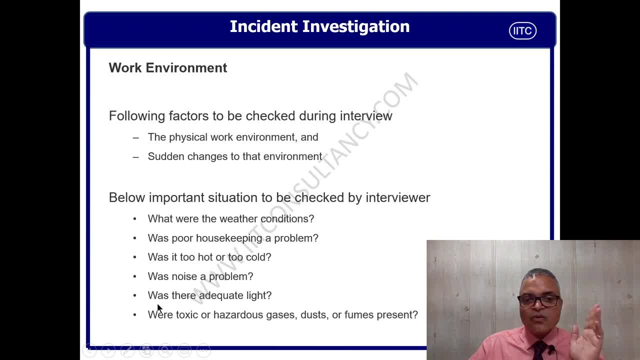 Or very low? Was there a noise pollution? Was there adequate lighting illuminations? Were toxic or hazardous gas, dust or fumes present? See, sometimes toxic gases can also create an accident. You never know. These all have to be checked and asked by the interviewer to identify the right root cause of an accident. 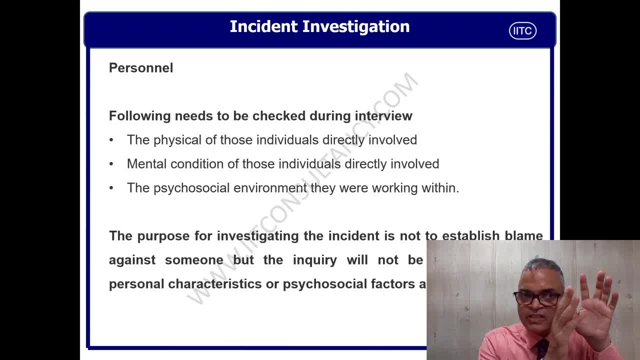 Following needs to be checked during the interview In terms of personnel. we have seen task material and we have seen other things We are going to see the personnel requirement. Following needs to be checked while doing the interview: The physical of those individuals directly involved. The physical condition of every individual who are directly involved in incident. 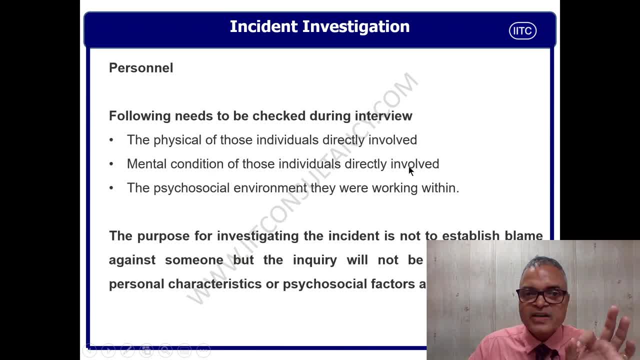 Mental condition of every individual who were directly involved. Psychological environment of the working place. So purpose of the investigation: the incident is not to establish blame against someone. But the injury will not to complete unless personal characteristics or psychological factors are considered. Incident investigation is not meaning to blame someone. 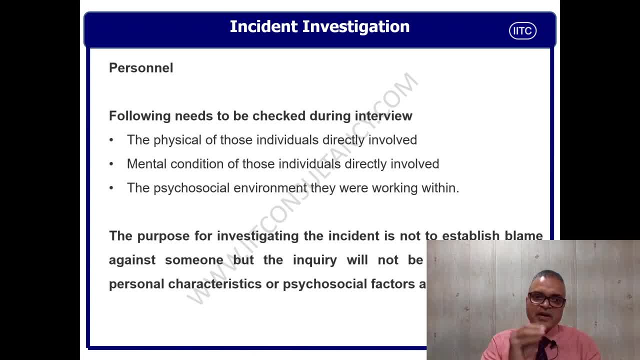 But until and unless we ask this question- physical condition of individual, mental condition of individual or psychological working condition- We are not able to identify right root cause of an accident. Accident investigation does not mean it is a blame game. No, We should not have a blame game while doing the investigation. 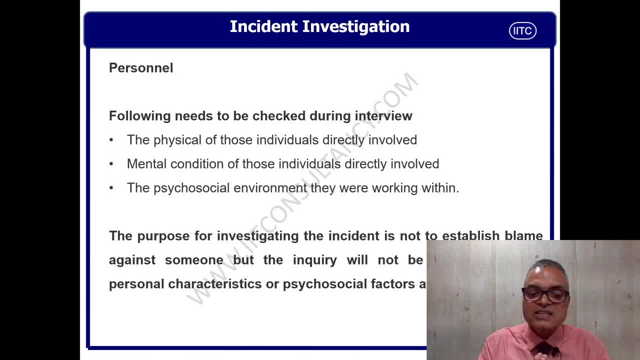 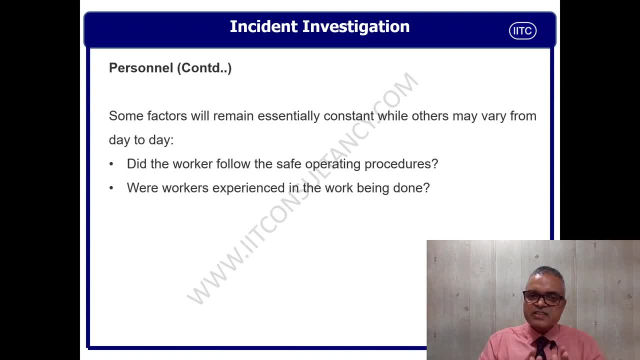 Or we should not understand. this is a blame game. This is not right safety culture. The right safety culture is to have a positive safety investigation. Some factors will remain essentially constant while doing the investigation, But some questions may change. These questions may be customized or should be customized. 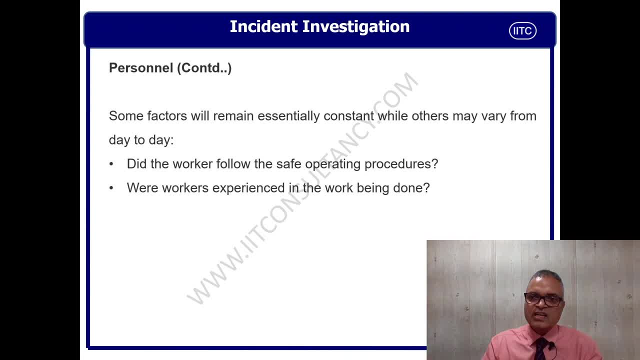 Depending on your requirement, Depending on your processes, Depending on your legal requirements. Depending on your legal requirements, Depending on your government, Depending on your working condition, Depending on your safety rule, Depending on your procedures. But some essential questions are there. Did worker follow the safe operating procedure? 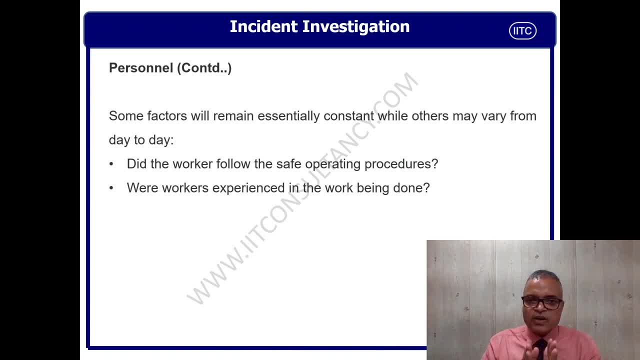 This is standard question to be asked Where worker experienced in the work being done, Whether the person is old person- Was he trained on doing this kind of job- Or this person is new, Whether the induction was done. So these are typical standard questions while doing the investigation. 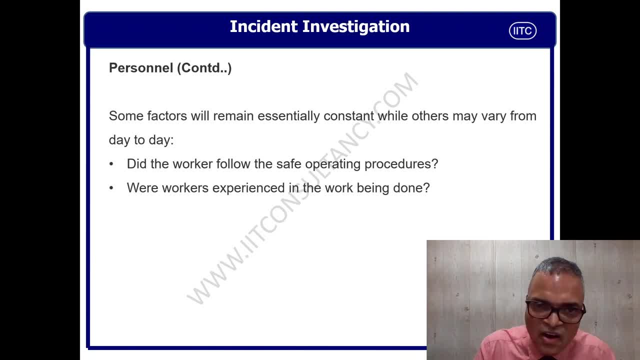 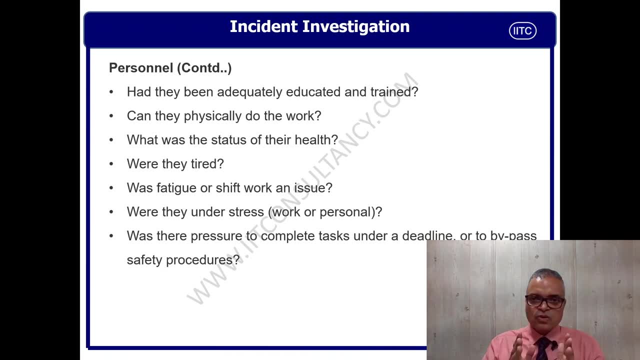 To find out the right root cause of an accident. Had they been adequately educated or trained? Whether person is old or educated and trained of doing the same job where the incident happened, Can they physically do the work? So we need to identify whether this job can be done physically. 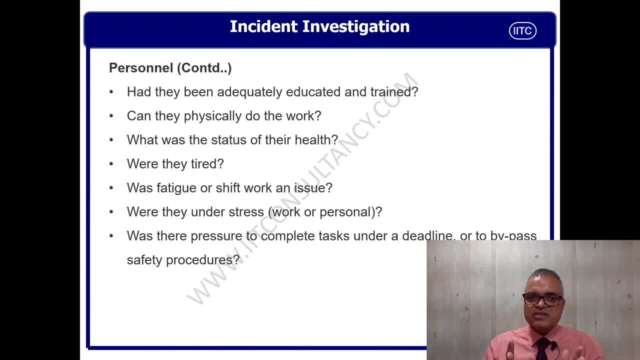 Or are they capable of doing this job physically? What was the status of their health when the incident happened? Was he sick, Was he comfortable, Were they tired Or they were doing overtime? They were exerted, They were having stress. Was fatigue or shift work as an issue? 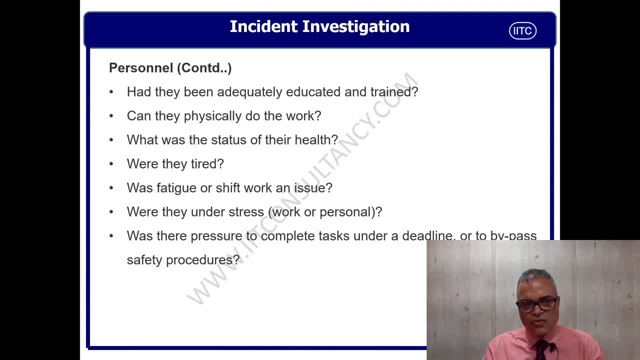 Was this incident happened in the night? Was there shift incident? Was they tired Or they were doing the work from more than 8 hours, More than 16 hours, More than 24 hours? But although this is legally prohibited To give overtime. 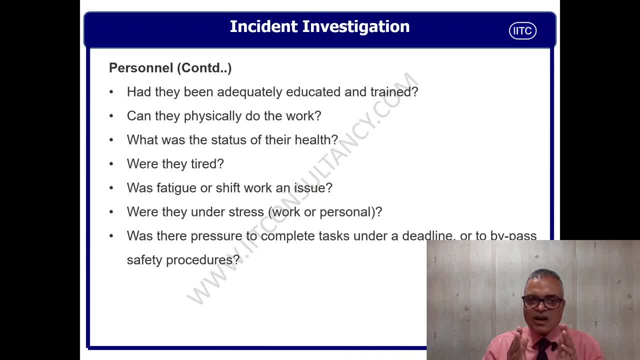 To prevent human stress. Were they under stress? So work stress or personal stress? Whether they were stressed to complete the work in given time Or they were under personal stress, Was there pressure to complete the task under a deadline Or to bypass any safety procedure? 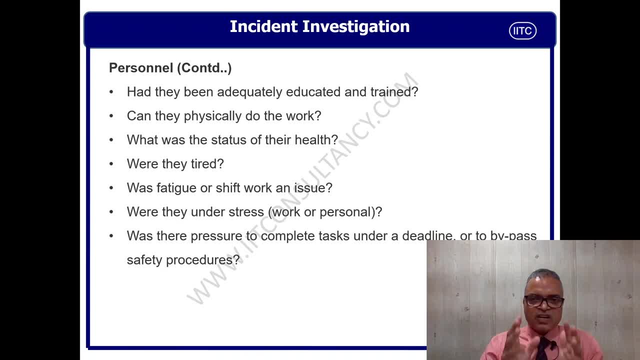 So these all points are very credible and important points. I would request you guys to please take a note While you are doing the investigation. These questions are guidelines only. You can customize these guidelines depending on your requirement. These are the standard questions. 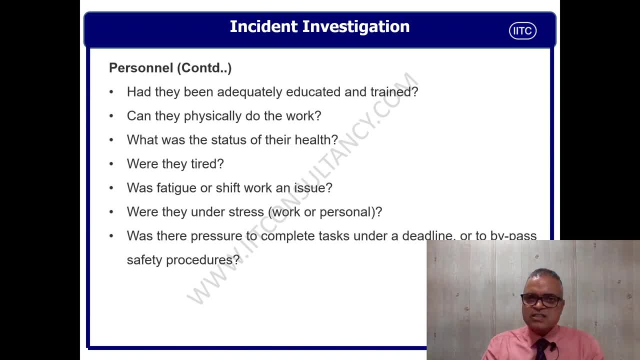 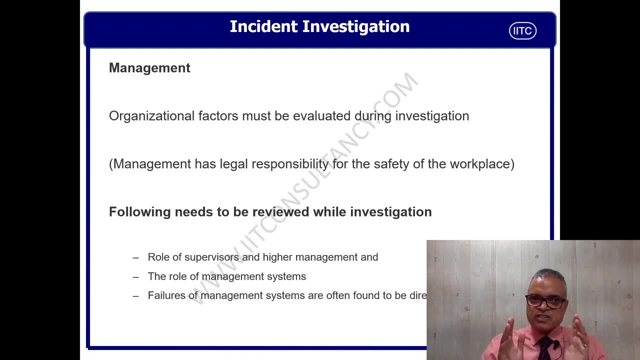 It will probably not change, But if you feel that there is change, Please change it, Update it And use these questions as per your requirement. Guys, management factor or organizational factor must be evaluated during investigation. Organizational factors are very important Because management has legal responsibility to safety of the workplace. 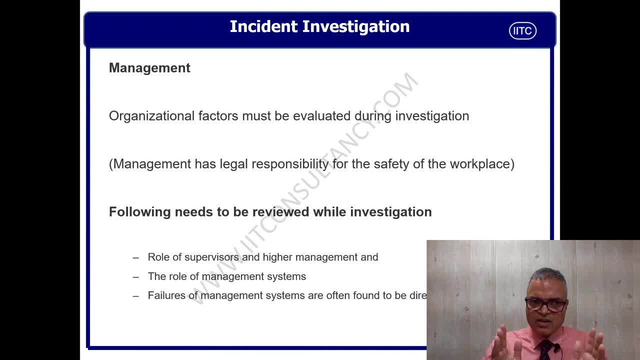 Ensure the safety of workplace, Ensure the safety of each individual. So we need to review following questions while investigation: The role of supervisor and higher management In this investigation On that day of investigation. Role of management system. What was the role of management system? 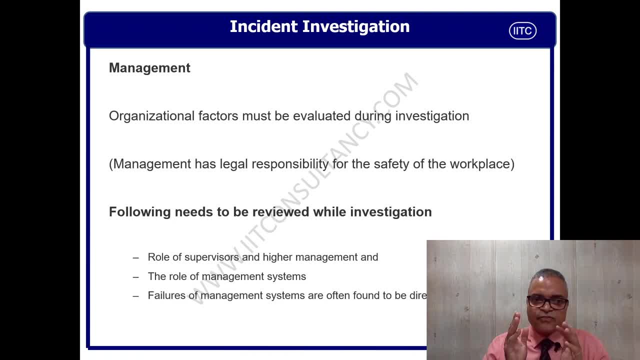 Whether the management knows the role And failure of management system are often found to be direct or indirect cause. Basically, if you see immediate cause, Basic cause and root cause, So ultimately the root causes goes to the management system failure. So we need to identify all the organizational factor. 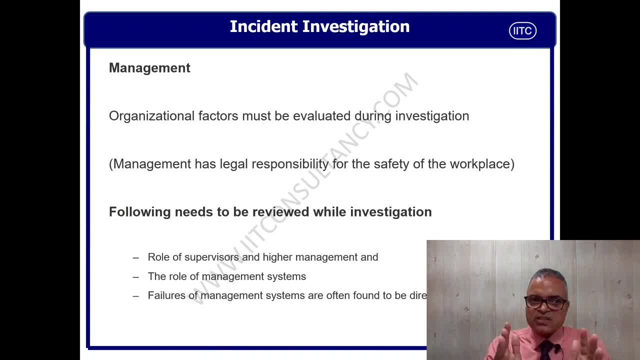 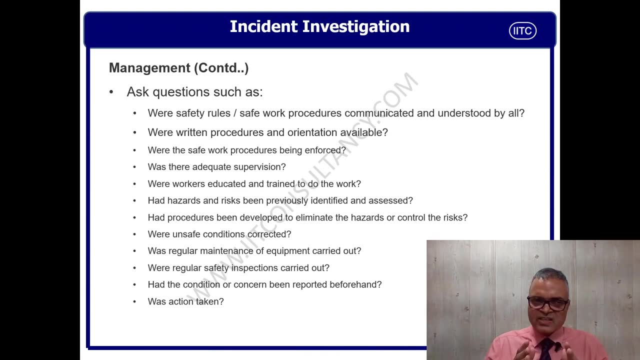 To evaluate the root causes, To find out the right root causes, Because management has role To identify and give the right shape working place to the worker While doing investigation. Let us go through the straight way. questions. I will not deliberate it. 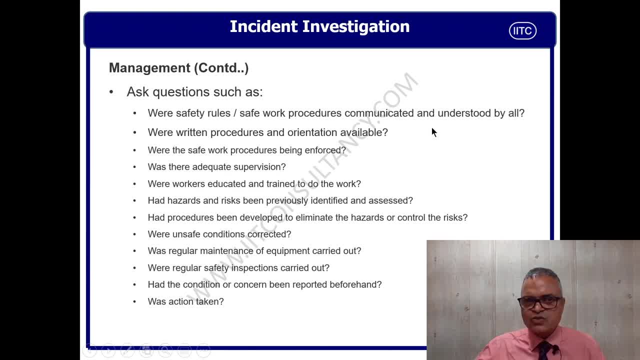 The safety rules and safe work practices communicated and understood by all Every person who is working in environment. He must be communicated the safe working procedure And he has to understand what is the meaning of safe working procedure And what is the meaning of unsafe act. 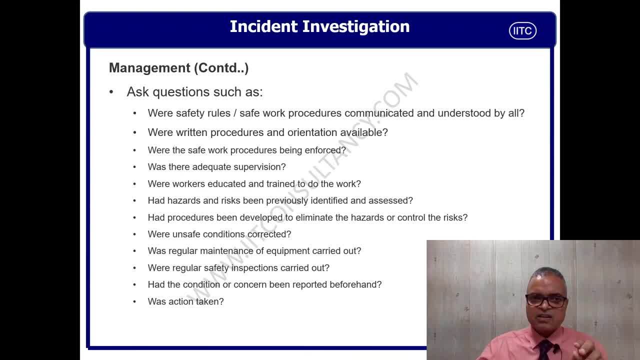 Unsafe condition And what are the various hazard in that work, Where written procedures and orientation available, Whether these people were inducted And whether the written procedures are in place, And whether these procedures are available in the local language Or these people understood. 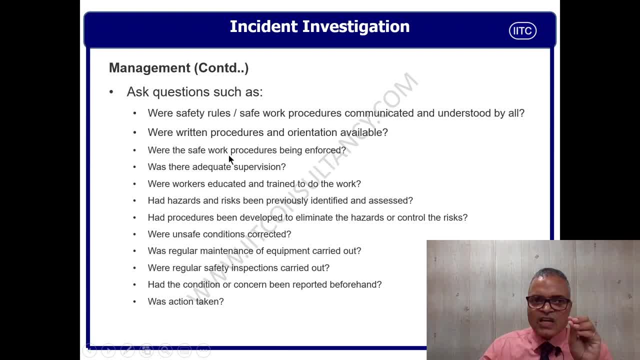 The procedures clearly Where the safe working procedure being enforced Or are you enforcing the safe working procedure And this is as per company rule? There may be not regulatory requirement, But this may be company rule. I do not know. You have to evaluate the factory act. 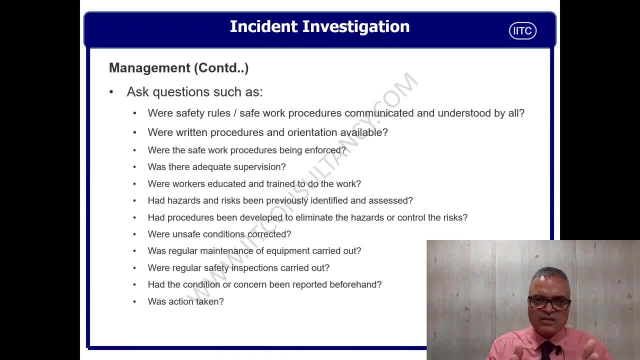 Environmental role And law of land As per your company situation, As per your company location? Was there suitable supervision Where supervisor in place, Whether supervisor knows Whether supervisor has given the LMRA Last minute risk assessment, Whether he has done the toolbox. 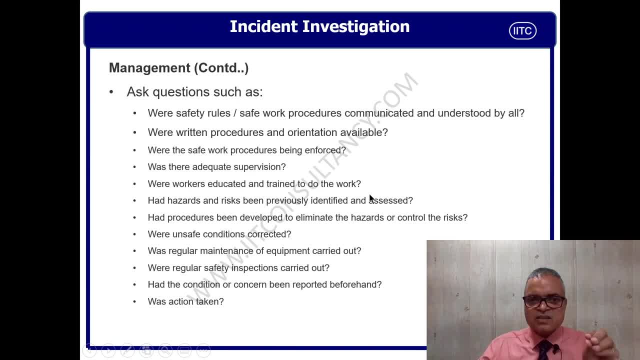 Where worker educated and trained to do the work, Whether those people who have been involved in the incident Have been trained Or they know how to do the work safely. Hazards and risk been properly identified and assessed, And control measures have been taken. 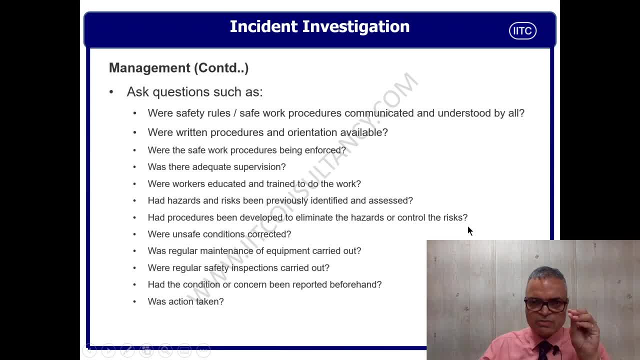 To eliminate the hazards So that hazards and risk can be minimized Where unsafe conditions correct If there were some unsafe condition, Whether unsafe condition corrected Was, regular maintenance of equipment has been carried out. If this job involves some hand tools, Some equipments. 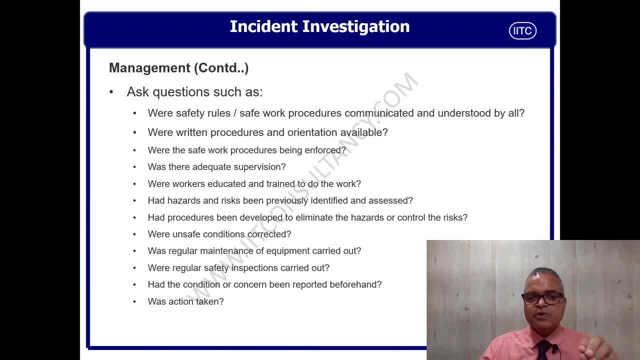 Whether the proper test was done, Whether the maintenance inspection was done on regular basis And whether that equipment is in functional condition. This all we have to identify in the interview Where regular safety inspection was done For that job, Near that job. 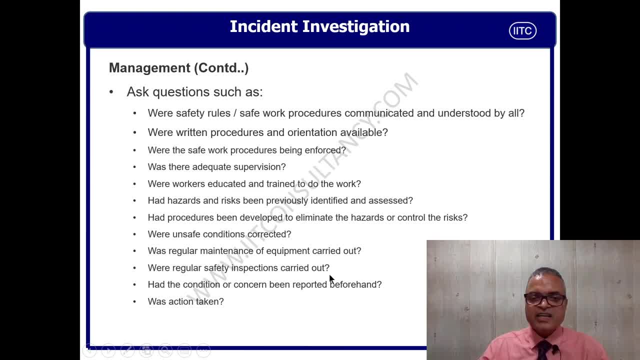 Near the work place, Near the equipment. If the hazard is identified, Whether the hazard has been removed. Has the condition or concern been reported? Reported, If there is unsafe condition or unsafe action, Whether those conditions or actions have been reported. Was action taken? 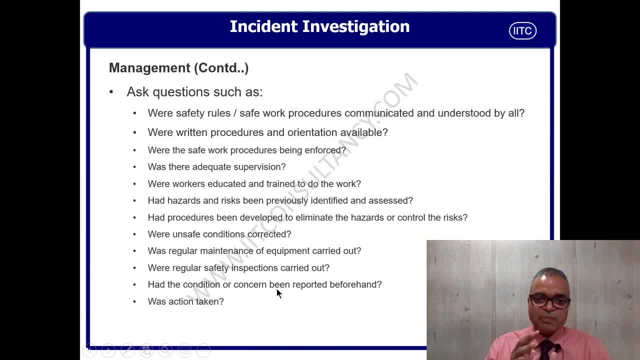 After reporting an unsafe condition, After reporting an unsafe action, Whether the safe control action measure has been taken or not. So, guys, these all questions are not general questions. These questions are applicable almost in all accident, But you feel free to Feel free to customize these questions. 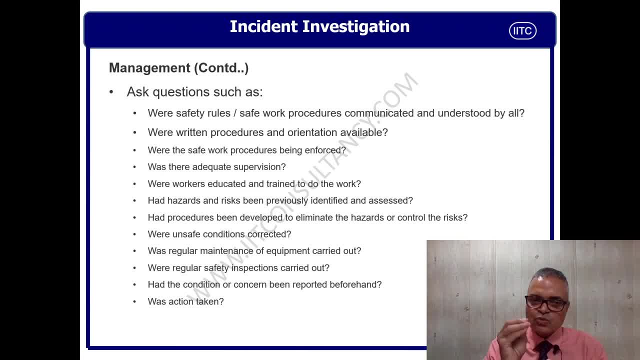 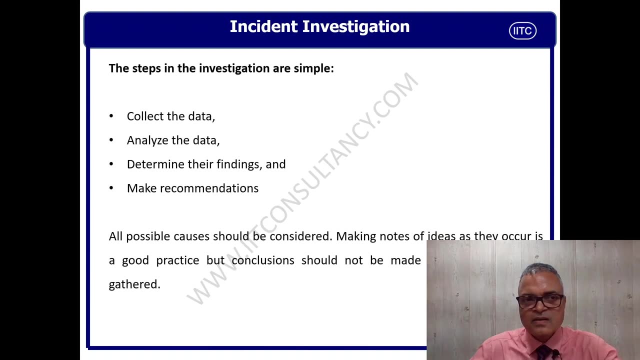 So that you can ask a right question To right person at right place, To identify the right root causes, To identify right control measures, To implement right control measures So our intention to prevent the incident can be achieved. So, guys, I mean, as we know that there are various steps in the investigation- 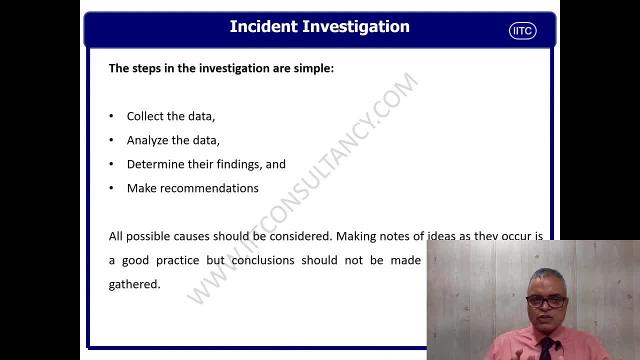 Collect the data of the incident, Beginning from the securing the work place- I mean incident place, Taking the photographs And doing some collection of other data. Analyze the data in various aspects: Working environment, Working condition, Work stress, Human. 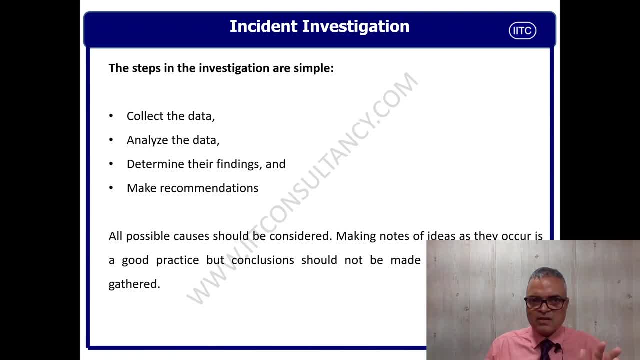 Man Machine Material In all aspects, The past history, Legal requirement, Training, data, Age of people- Everything has to be determined. I will not narrate the list of questions that have to be analyzed, But you feel free to ask me any question. 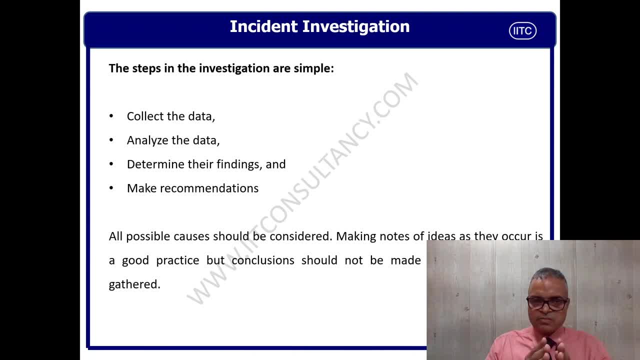 In the comment section. If you want some list, I have prepared excel sheet. I can put this excel sheet in the description box. You can download this checklist for doing the data analysis during investigation. Determine their findings, Make recommendations. All possible causes should be considered. 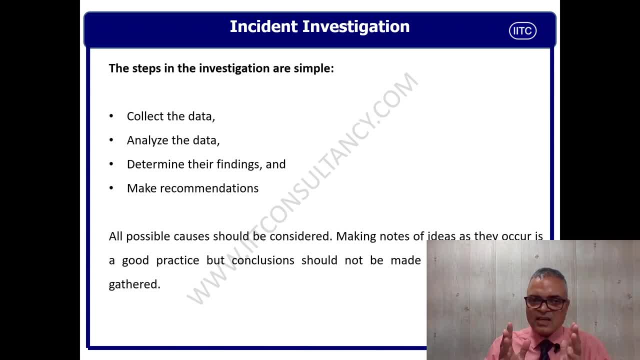 Making notes of idea as they occur is a good practice, But conclusion should not be made until all the data is gathered. This is very important. Do not do half fry. Do always complete cooking Without the data or in absence of all the data. 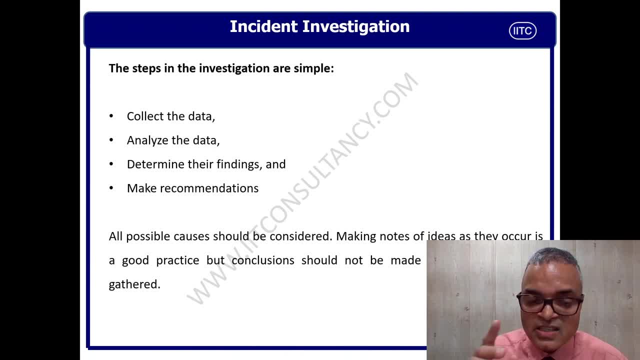 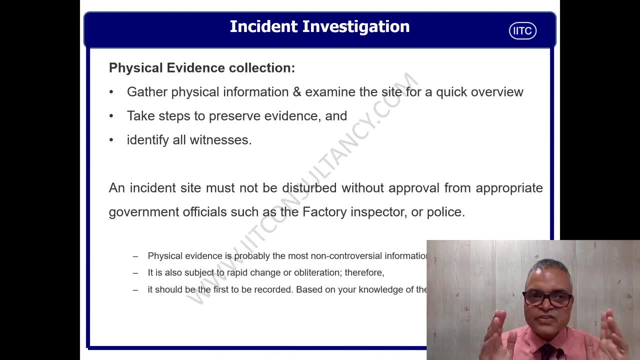 Please do not start the investigation Because this can be hazardous. This can guide you. This can misguide you. Ultimately, we cannot find out the right root causes. Physical evidences are very much important. Gather physical information And examine the site for work. 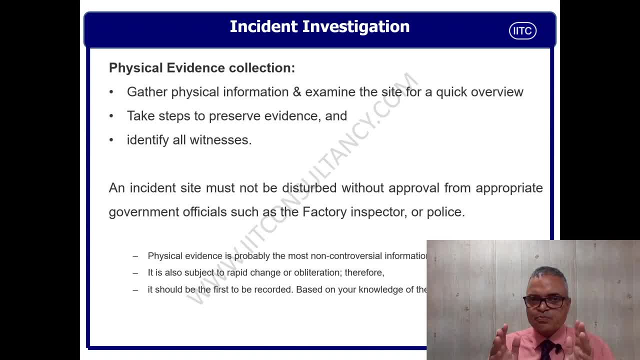 For quick review. Take steps. Take steps to preserve the evidences And identify all witnesses, As you know that if you do not identify the physical evidences, If you do not secure the physical evidences, Probably this will go very quickly. 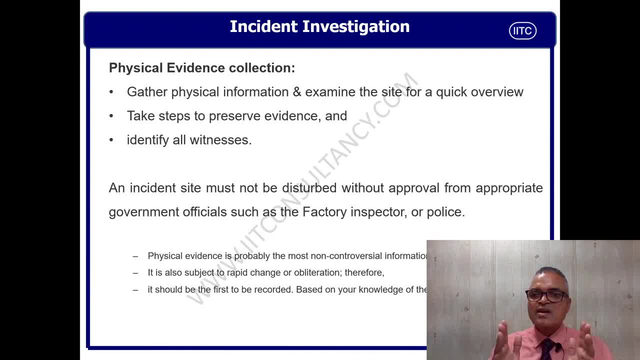 An accident. site must not be disturbed without approval from appropriate government officials, Such as factory inspector or people. Sometimes there is requirement. Site should not be disturbed. Evidences should not be destroyed. This must be secured. This is legal requirement. Factory inspector is. 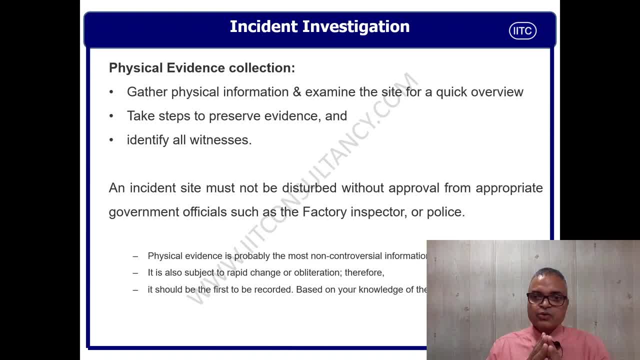 I mean authority to tell you You can disturb Or you can upset, You can remove Now the site After doing the investigation. Physical evidence is probably the most non-controversial information, Because physical condition is important to guide you what went wrong. 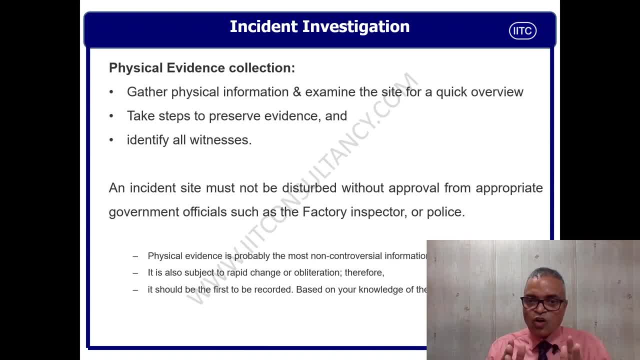 It is also subject to rapid change or obliteration, Because it will change very quickly. Some body will replace it, Some body will go and take something, Not intentionally, But because of housekeeping. Some housekeeping person will go and clean it. 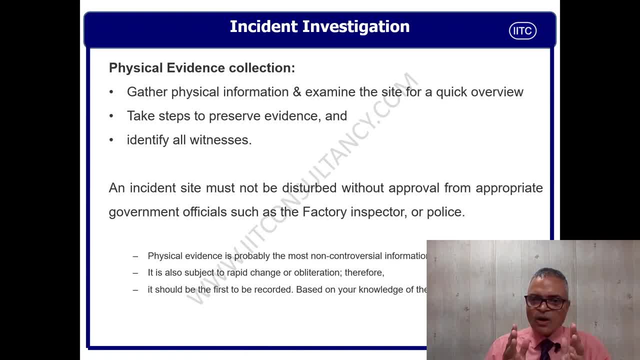 It should be first to be recorded, Based on your knowledge of the work processes. So, my friends, I would like to tell you my experience That if, in case of any accident, Secure the incident place immediately And try to take the photographs as much as you can do. 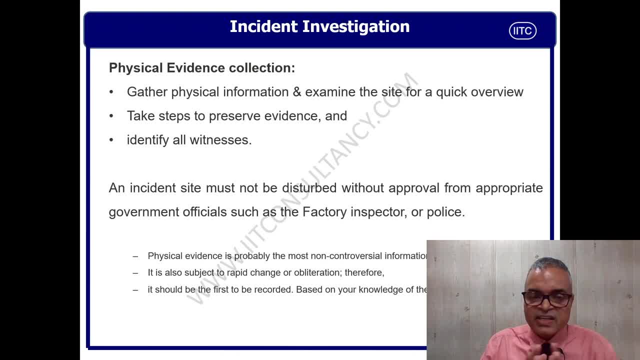 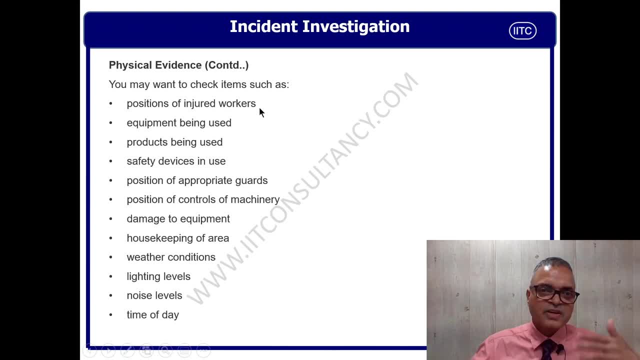 Otherwise the incident. root causes can be vanished, Can be removed. Physical evidences may be like this: Possession of injured worker. Probably the worker is not there, But you can simulate it. You can simulate how the worker was working, Equipment being used. 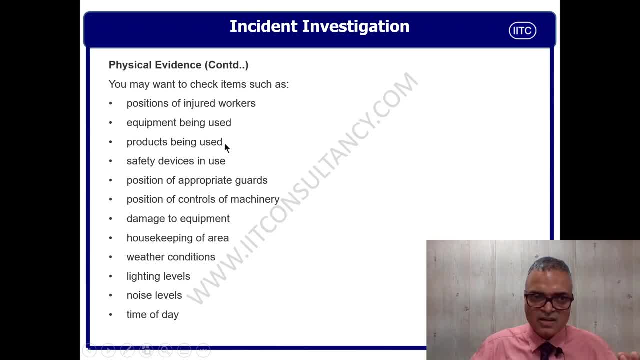 What equipment was being used. Product being used, Raw material, Process material Catalyst Must be analyzed. Safety devices in use, Any safeguard, Any safeguard, Any preventing safeguard, Mitigating safeguard, Controlling safeguard, Possession of appropriate guarding. 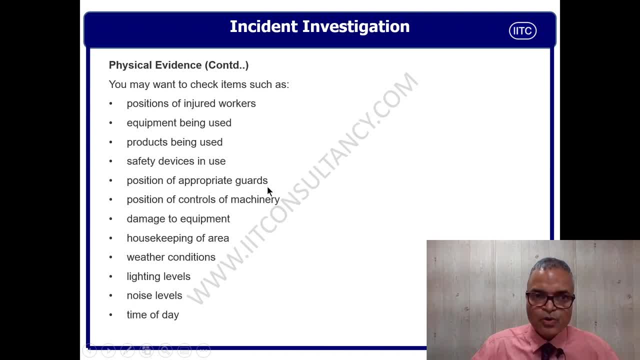 Whether guards were in right place. Right position, Appropriate guard was there? Sortable and sufficient number Control. Position of control of machines. What is the position of control of machinery? Damage to the equipment: What was the damage? Extent of damage. 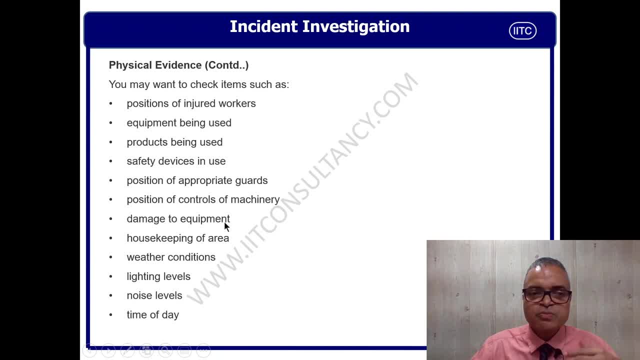 How it was damaged, Where it was damaged, What piece portion of equipment damaged. Take the photographs. How skipping of the area To avoid any. I mean unsafe act or unsafe condition. Any unsafe condition like slip and trip and other things. Weather condition. 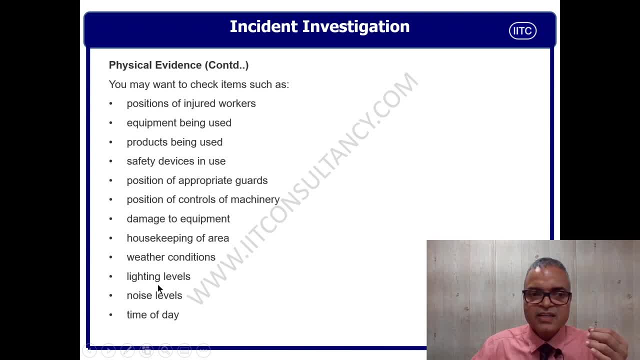 What was the temperature, What was the noise, What was the illumination, Lighting levels, Noise levels, Time of the day When it happened? In day shift, In the night shift, During shift. So these points must be considered while doing the investigation. 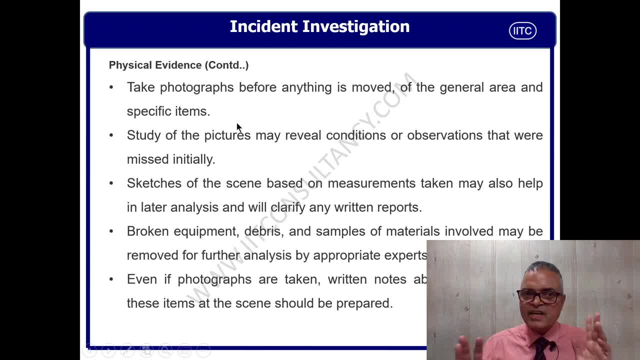 And physical evidences. Take the photographs before anything is moved, Because if you don't take the photograph probably you will be misguided. Study of the pictures may reveal the real condition of the incident. Sketches of the scene based on the measurement can also be useful doing investigation at. 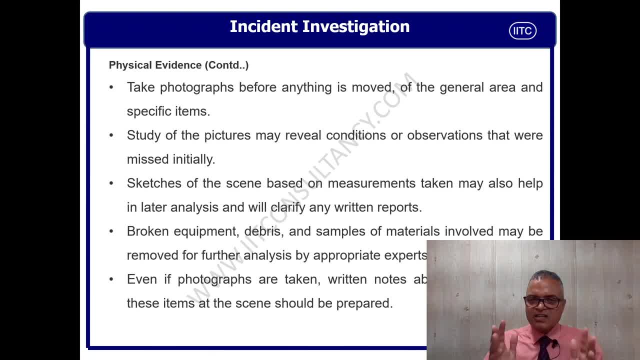 the latest stage, Broken equipment, Debris, Sample of material involved in the investigation in the incident should not be removed. It must be analyzed to identify the right root cause. Even if the photographs are taken, written notes must be put during the site visit. 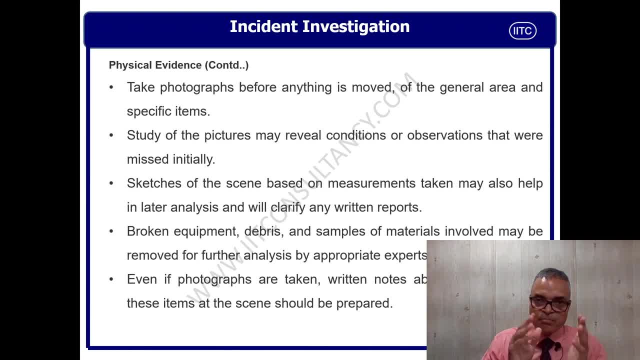 During the evidence check, During securing of evidence. These points are very important to give you clear, cut root causes. Don't stare at the legal requirement. Don't even try to demolish or remove anything involved in the incident, Because this is the legal requirement. 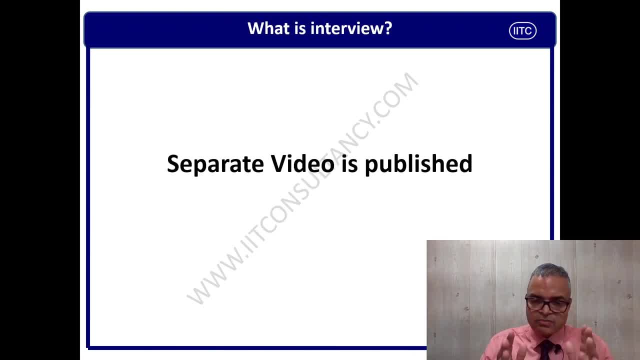 Not to be tampered. So, guys, I mean, having known all these questions related to man, machine, material management and system and equipment, You can customize your question Depending on your suitability, Depending on your work, Your working environment, Your procedure. 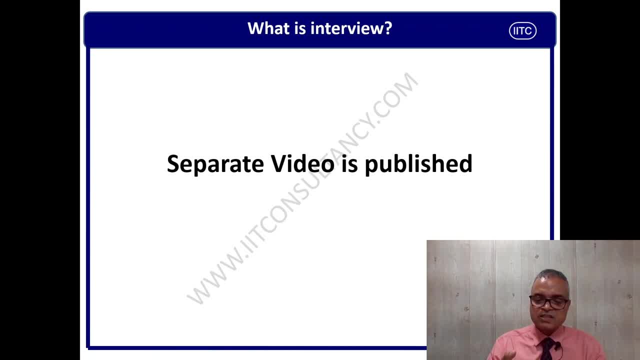 Your processes, Legal requirement, Management expectation. About your incident investigation procedure, I have casted a separate video How to do interview, Who to be interviewed, What are the techniques of interview? I mean, what are the do's and don'ts of interview? 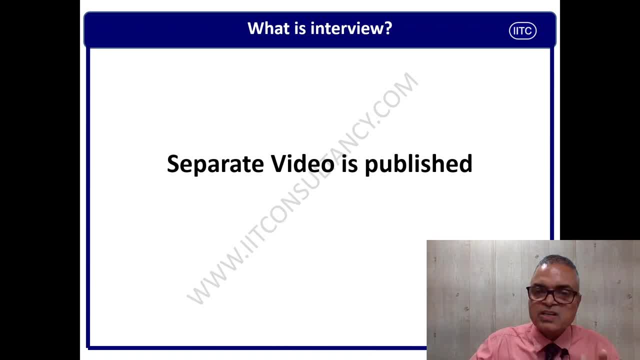 I would request you to guys, please see this video to understand the complete information of interview techniques. I will not take much time of yours to tell you what are the incident investigation techniques, How to do the interview. You can do it later on as per requirement. 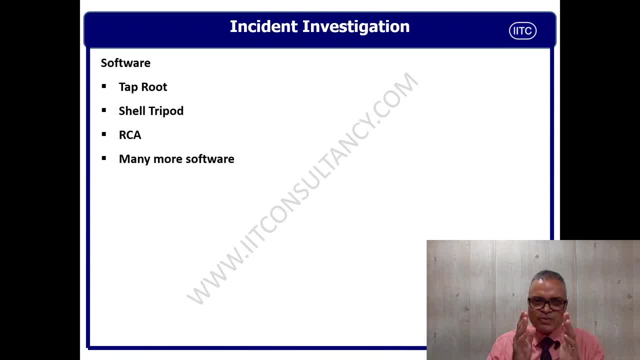 As we mentioned that we will see the investigation softwares. There are some softwares on which I am trained, I am skilled. I know TEPRUT, I know CELTRAPOID, RCA And many other softwares like YY analysis. 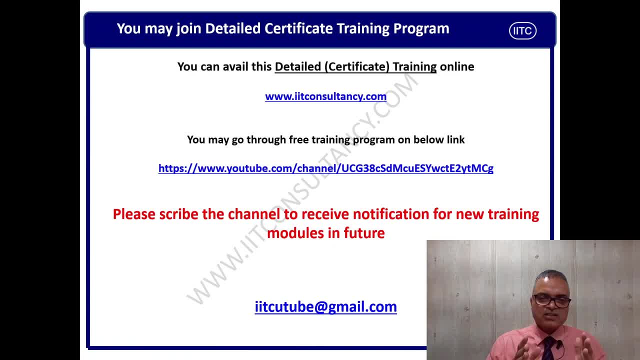 FISBOT techniques Guys, I hope this was this incident investigation Presentation was useful for you And let me know if you have any question in the comment section With this guy. I would encourage you to please see other videos relevant to the incident investigation. 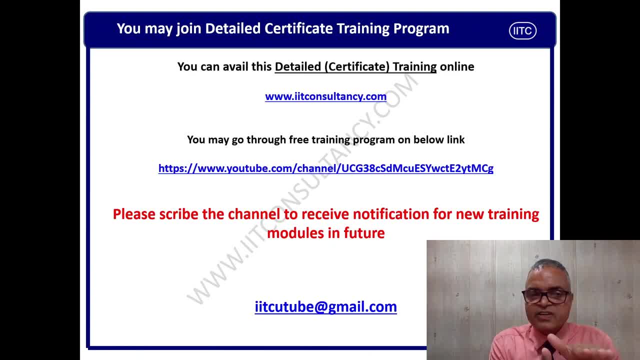 Because there are other 4 to 5 videos relevant to safety incident investigation Which will give complete idea So that you can do your investigation unbiased way. You can find out the right root cause, You can find out right recommendation, You can implement right recommendation. 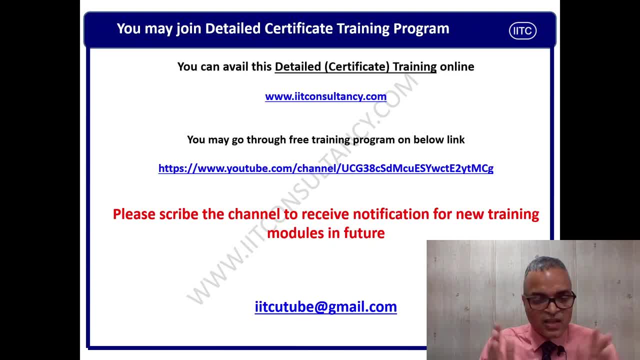 Which can prevent re occurrences of this incident. Guys, with this, thank you very much. Have a nice day. Jai Hind, Jai Bharat.